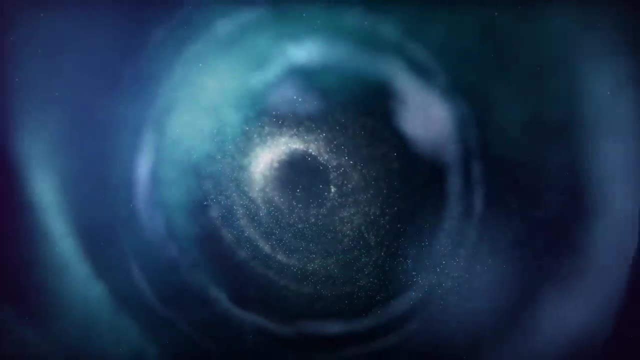 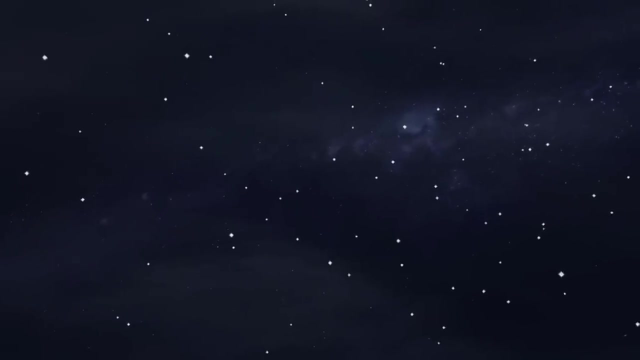 need to uncover the most fundamental laws and determine how they act on the finest constituents of matter. Thankfully, this universe is not our universe. If it were, it's hard to see how science would have made any progress at all Over the centuries. the reason we've 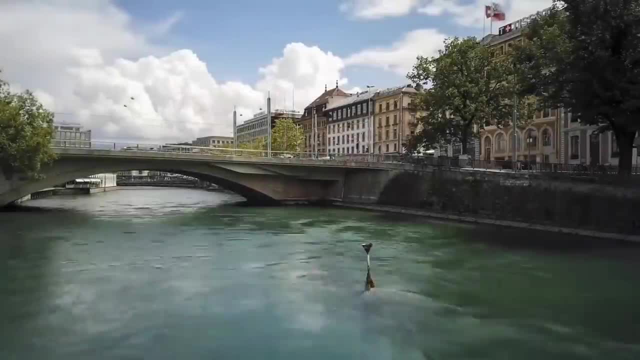 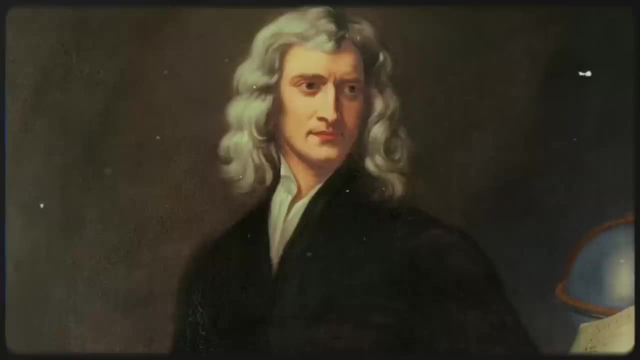 been able to make headway is that we've been able to work piecemeal. We've been able to unravel mysteries step by step, with each new discovery going a bit deeper than the previous. Newton didn't need to know about atoms to make great strides in understanding. 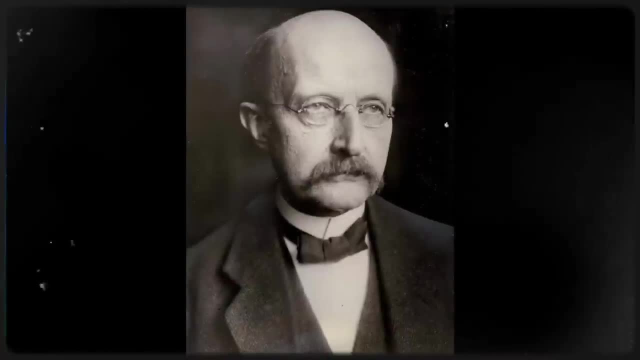 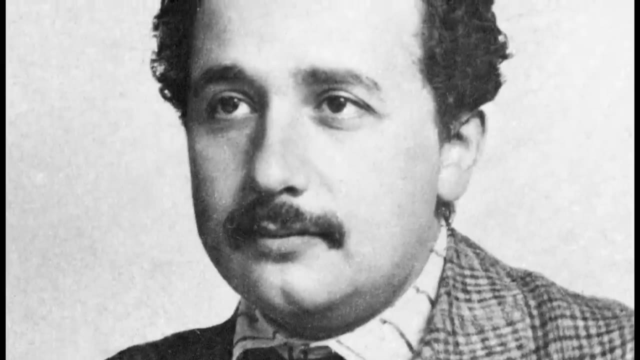 motion and gravity. Maxwell didn't need to know about electrons and other charged particles to develop a powerful theory of electromagnetism. Einstein didn't need to know about the universe. He didn't need to address the primordial incarnation of space and time to formulate. 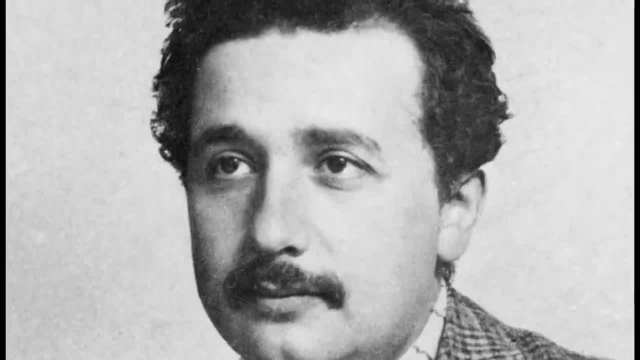 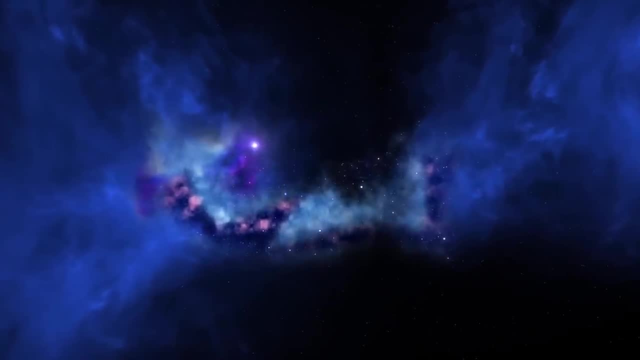 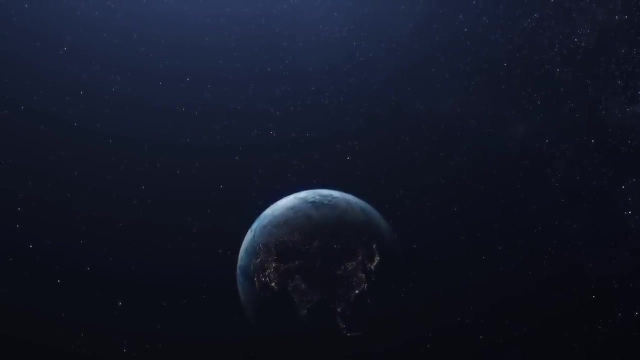 a theory of how they curve in the service of the gravitational force. Instead, each of these discoveries, as well as the many others that underlie our current conception of the cosmos, proceeded within a limited context that unabashedly left many basic questions unanswered. Each discovery was able to contribute its own piece to the puzzle, even though no. 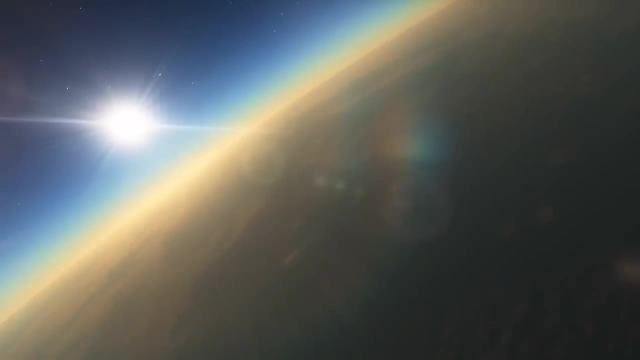 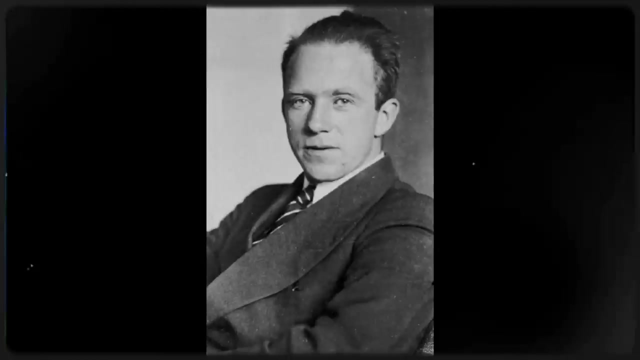 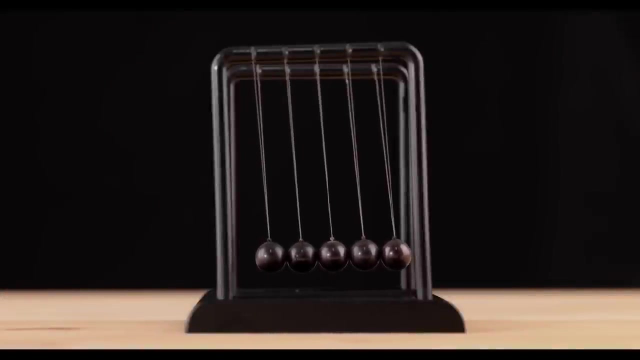 one knew, and we still don't know what grand synthesis it will bring. The uncertainty principle is one of the most evocative features of quantum mechanics, marking a significant departure from classical physics. Classical physics aim to describe physical reality by specifying the positions and velocities of all matter, constituents, as well as the 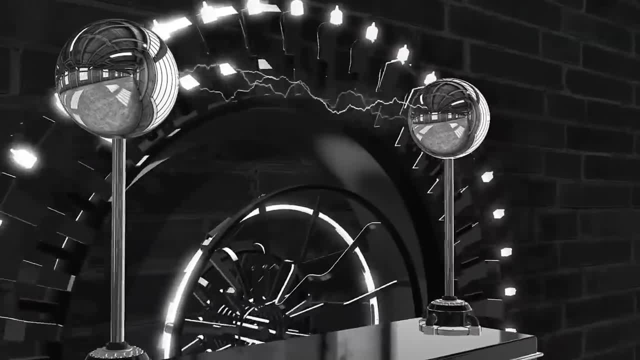 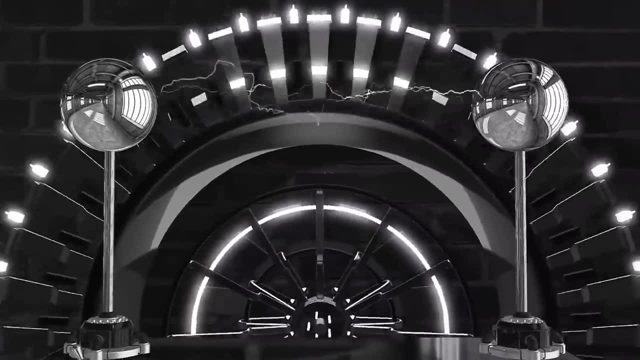 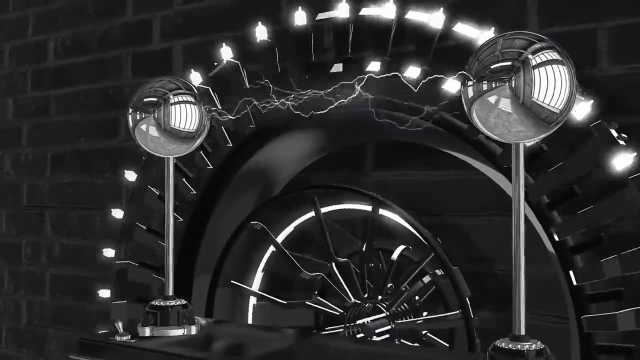 values and changes in values of each field, including electromagnetic and gravitational fields. In the 1930s, the uncertainty principle challenged this classical view by stating that it's impossible to know both the position and velocity of a particle simultaneously, or both the value of a field and the rate of change of that value. Quantum uncertainty. 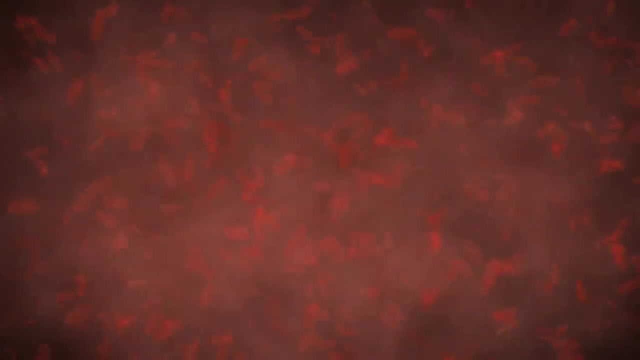 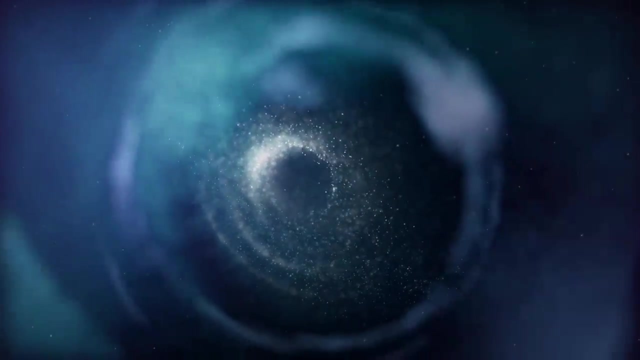 leads to a turbulent and jittery nature in the microworld, affecting all fields, including electromagnetic, strong and weak nuclear forces and gravitational fields. Quantum uncertainty is a very common phenomenon in quantum physics. Even what appears to be empty space is subject to quantum jitters, challenging the classical notion of emptiness In classical physics. 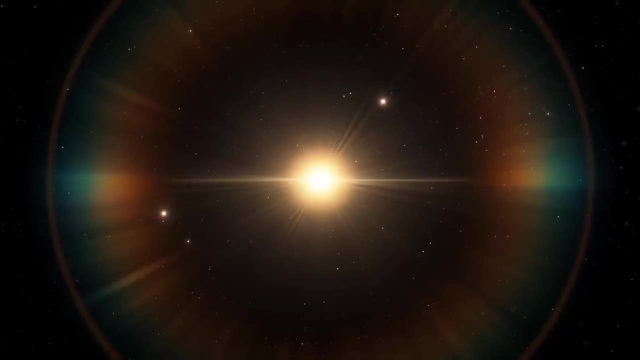 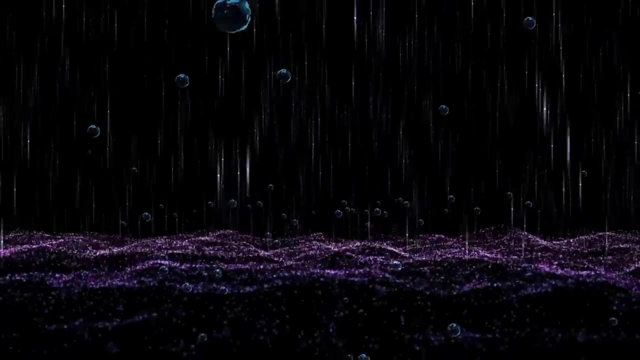 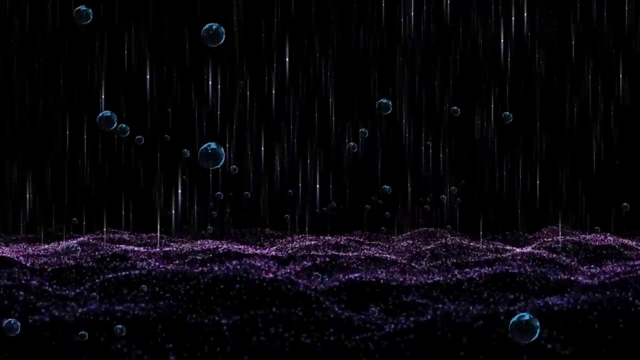 empty space was defined as a region with no particles and fields uniformly set to zero. However, quantum mechanics introduces the concept of vacuum fluctuations, where, even in empty space, fields exhibit random fluctuations in their values. The Casimir effect, discovered by Dutch physicist Hendrik Casimir, is a very common phenomenon in quantum physics. The 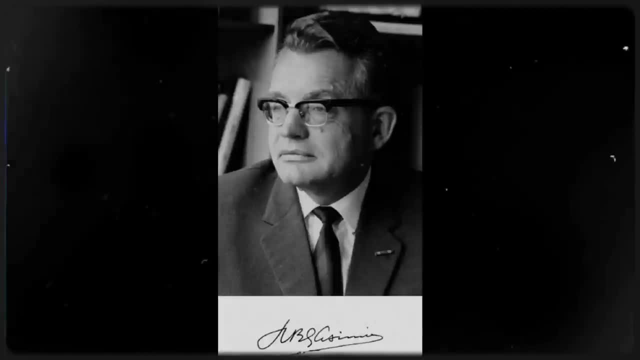 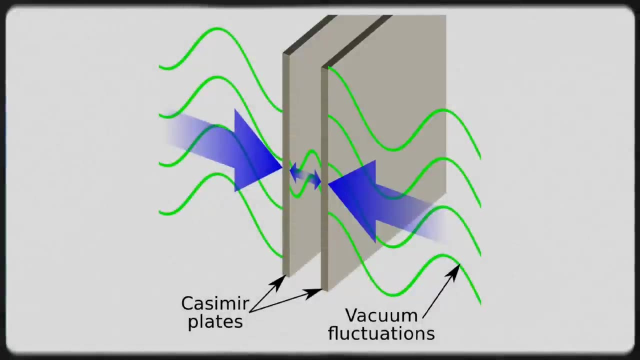 quantum mechanics. of quantum mechanics are the most common and most common phenomena in quantum physics. Casimir, in 1948, provided experimental evidence for vacuum fluctuations. Placing two metal plates in empty space led to a reduction in electromagnetic field fluctuations between the plates, creating a pressure imbalance that caused the plates to move closer together. 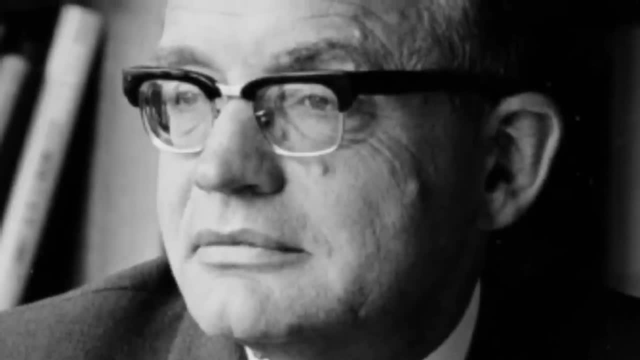 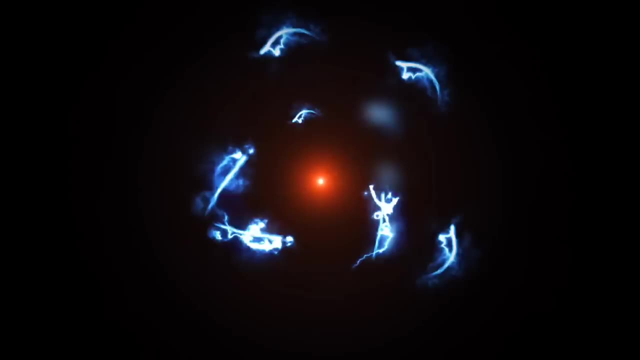 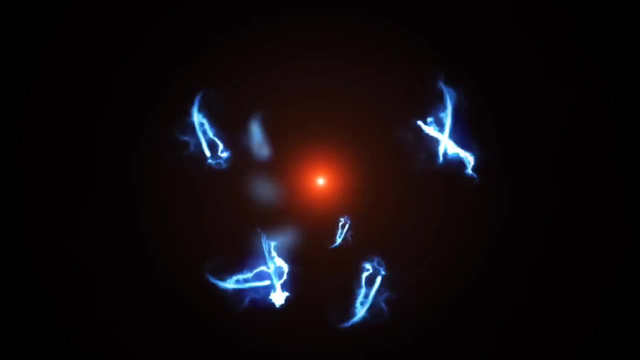 Casimir's theoretical predictions were later confirmed through experiments, demonstrating that empty space is not as static and eventless as previously thought. Quantum uncertainty, with its inherent field jitters, posed challenges to classical physics, but also laid the groundwork for modern quantum field theory, providing precise mathematical frameworks for describing 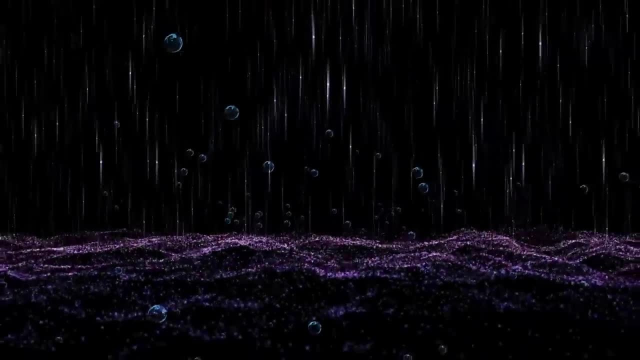 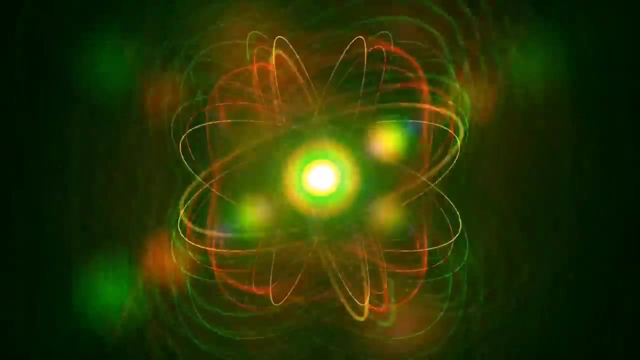 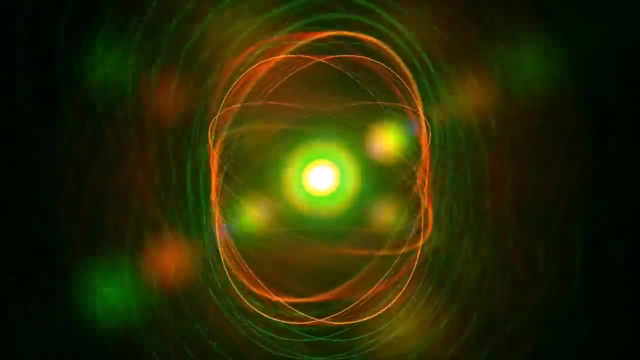 field fluctuations and their effects. The passage discusses the quantum jitters of space itself, which is an example of quantum field jitters. According to Einstein's general theory of relativity, gravitational fields are described as warps and curves in the fabric of space – and gravity of mountains. Mullten, McDonahan, Russell and Hamilton are talking. 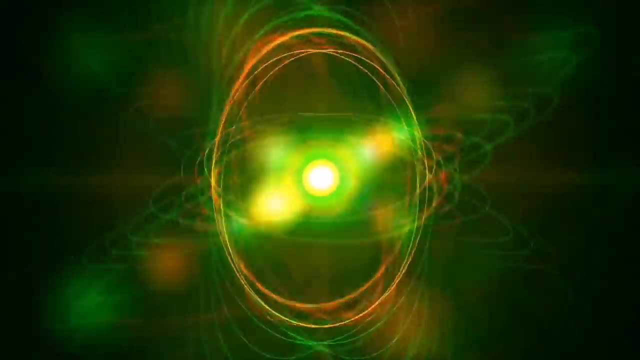 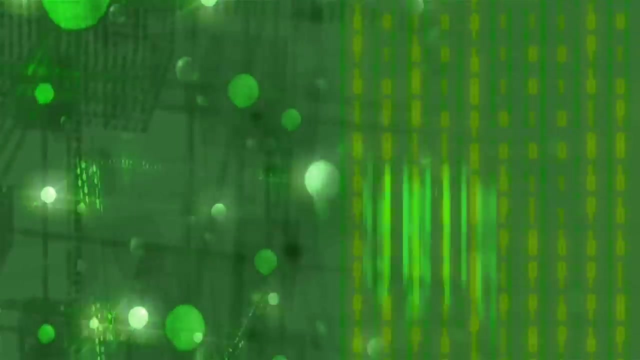 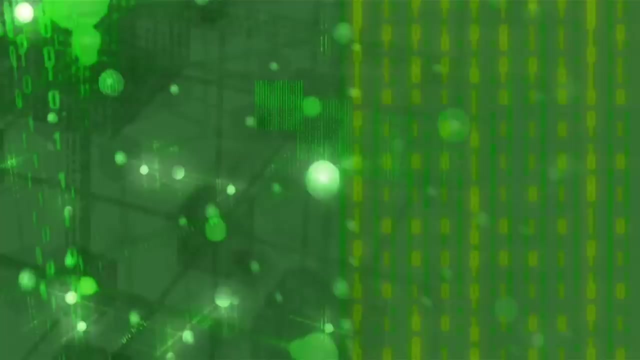 meaning that the shape or geometry of space itself is affected by gravitational forces. The uncertainty principle applies to the gravitational field leading to quantum jitters in the fabric of space. These jitters cause the shape of space to fluctuate randomly on tiny distance scales. 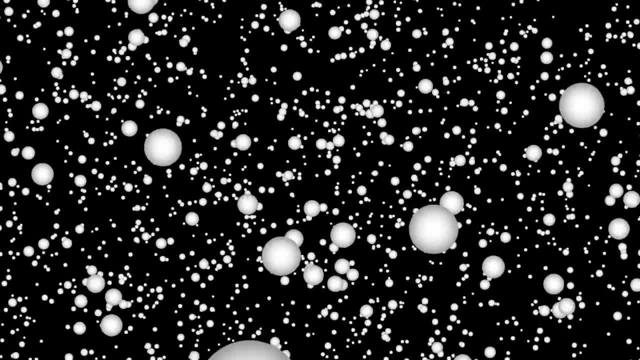 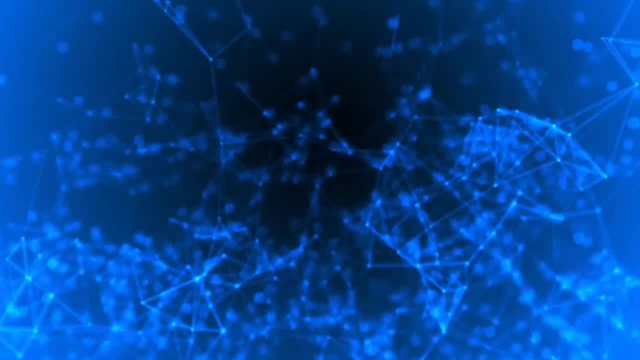 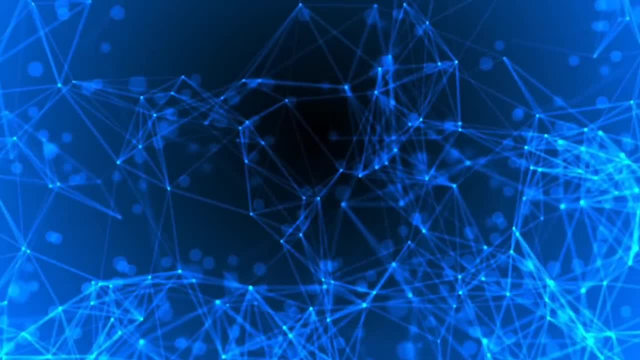 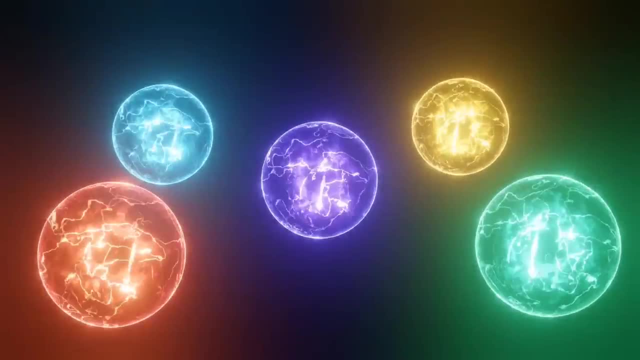 At everyday distance scales, the quantum fluctuations are too small to be directly observed and space appears calm and flat. However, as the observation scale is sequentially magnified, the quantum fluctuations in space become increasingly frenetic and chaotic. At scales smaller than the Planck length- about 10 circumflex, 33 cm- space becomes extremely turbulent and distorted. 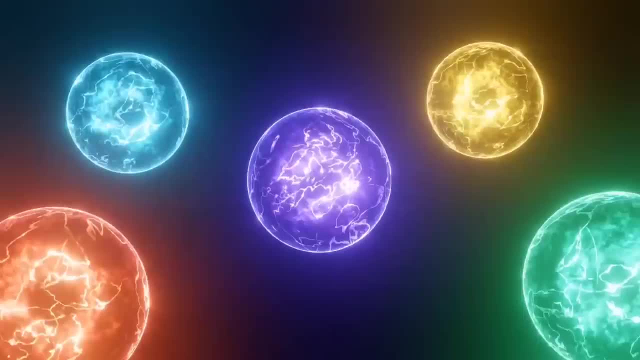 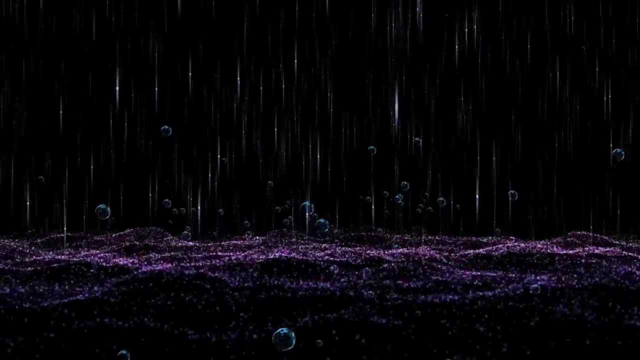 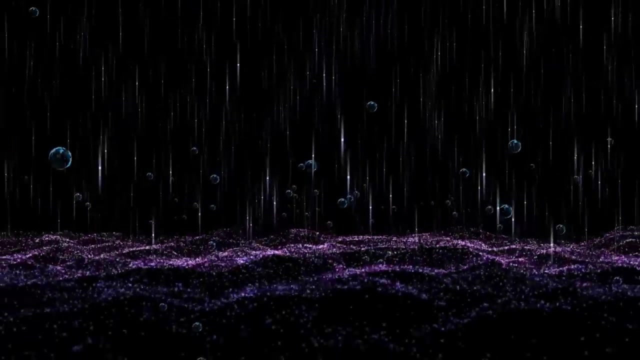 making conventional notions of left-right, back-forth, up-down and before-after meaningless. Quantum uncertainty on such small scales makes the usual concepts of space and time inapplicable, leading to a breakdown of Einstein's smooth and gently curving geometrical space. 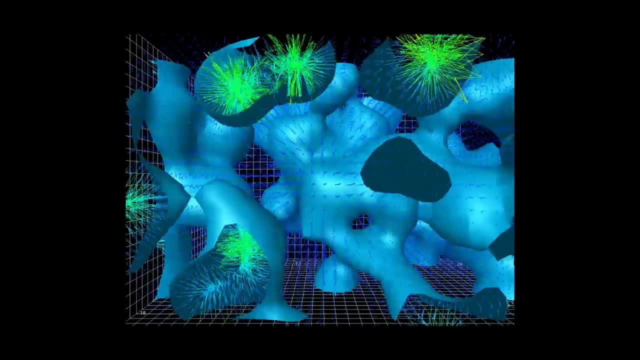 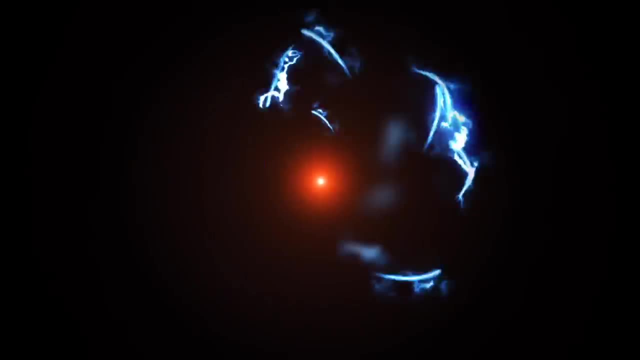 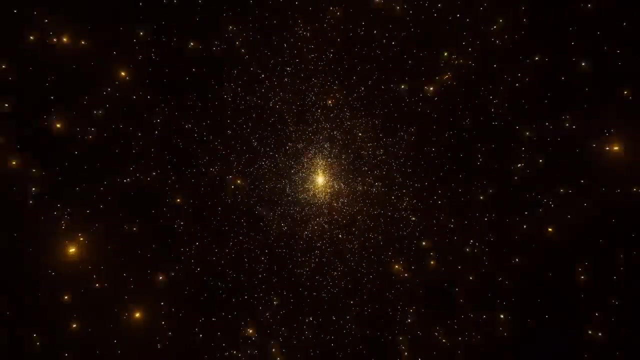 This emphasises the clash between the smooth spacetime described by general relativity and the turbulent, jittery nature of quantum mechanics, posing a significant challenge for physicists attempting to reconcile these two fundamental theories: The incompatibility between general relativity and quantum mechanics. 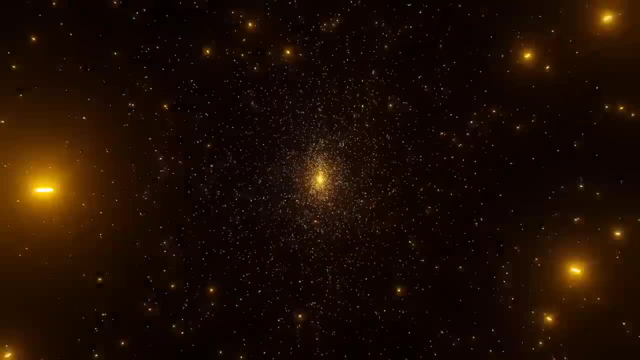 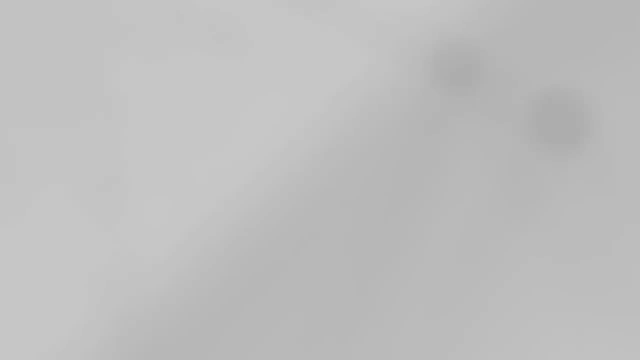 becomes ever more complex as time passes. It is evident when their combined equations almost always yield infinite results which are mathematically nonsensical and have no physical meaning. While special relativity and quantum mechanics coexist with some tension, their combined equations do not produce mathematical inconsistencies or meaningless results. 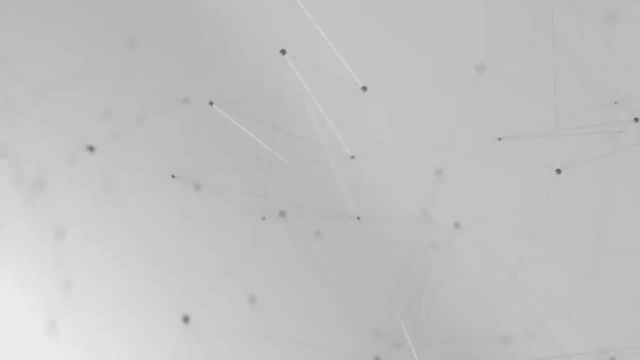 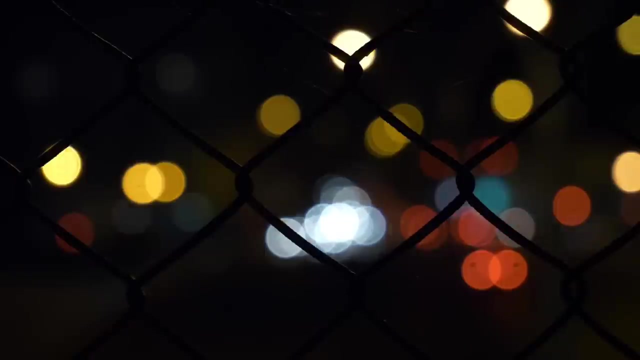 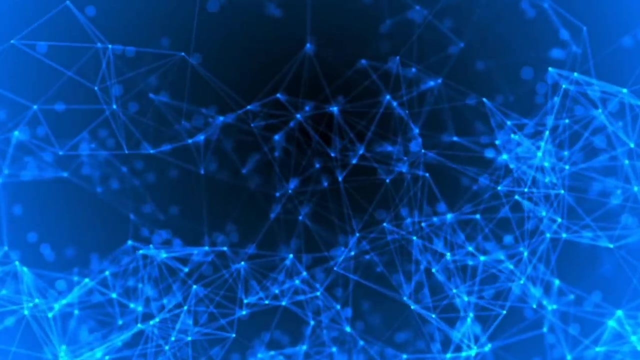 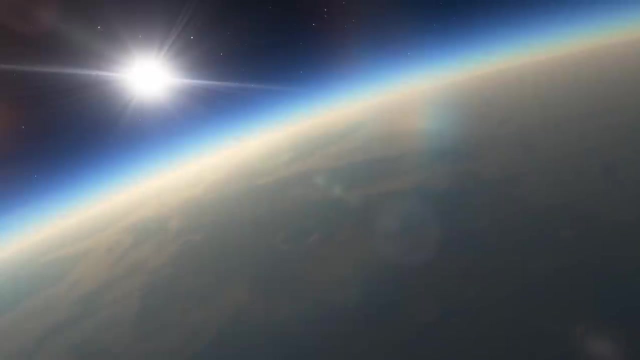 and have been used to make highly accurate predictions. Physicists have historically kept general relativity and quantum mechanics separate for practical purposes, with each theory applied to different scales of the universe. However, there are compelling reasons to reconcile these two theories. First, it seems artificial and unsatisfactory to divide the universe into two separate realms. 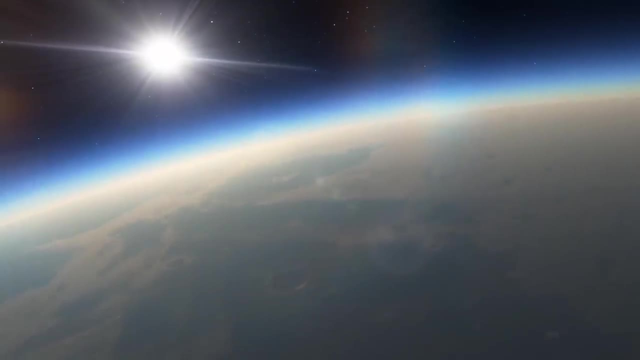 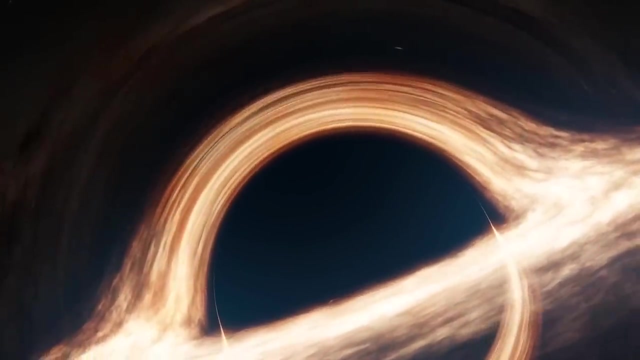 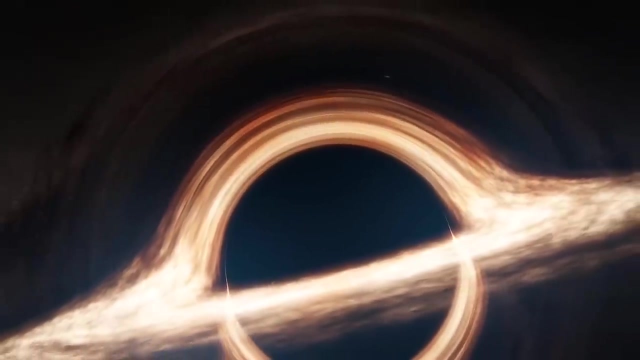 each governed by a different theory. Second, some physical phenomena, like the interior of black holes, require a unified framework as they fall into both the macro and micro domains where the two theories collide. Third, incomplete understanding of phenomena like black holes and the early universe. 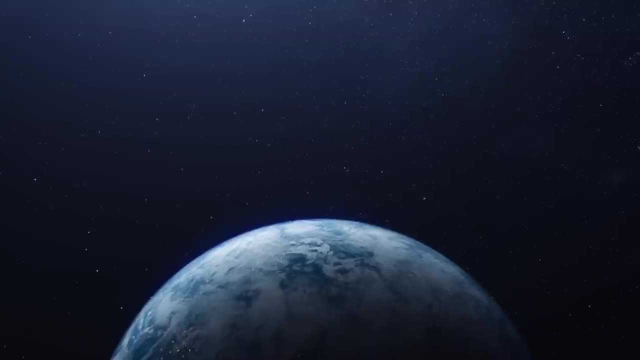 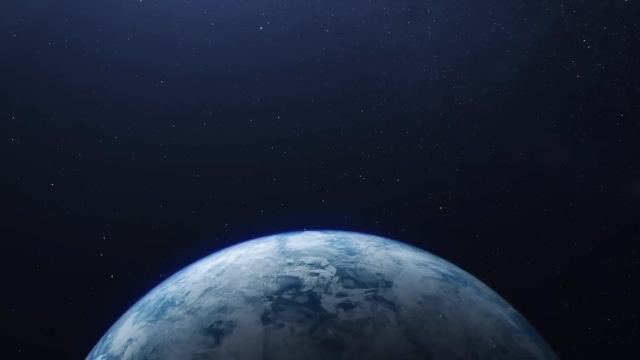 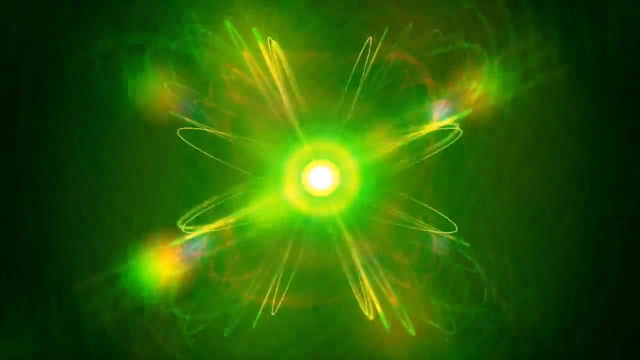 highlights the need for a unified theory to reach a deeper understanding of the cosmos. Resolving the conflict between general relativity and quantum mechanics is crucial for a complete understanding of the universe, especially regarding the origin and fundamental nature of space and time, which remains obscured. 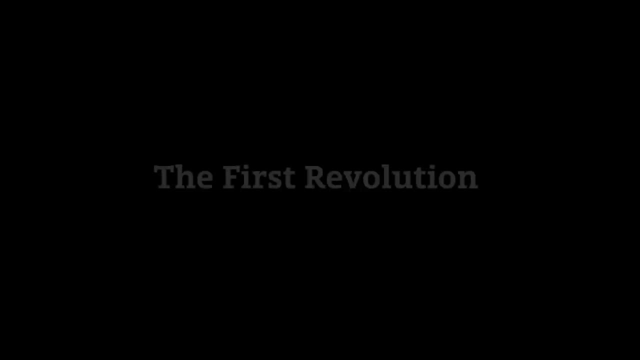 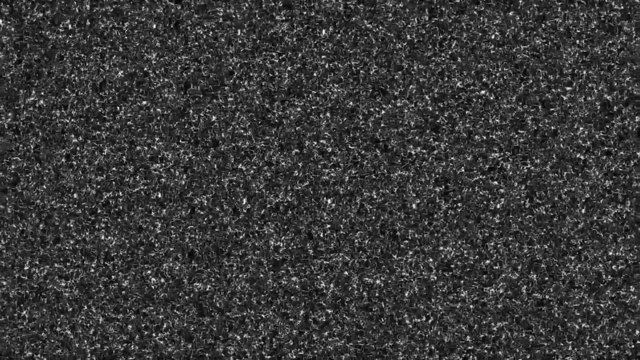 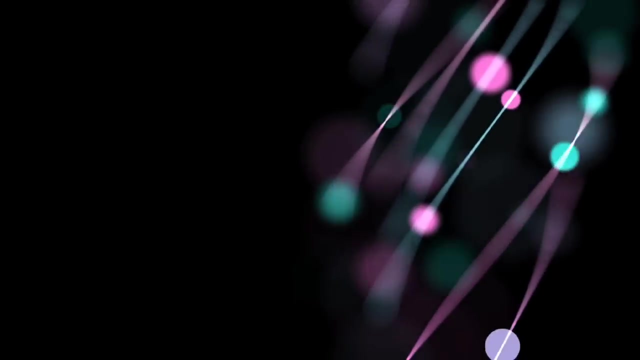 due to the unresolved conflict between the two theories. Superstring theory is an approach believed to merge general relativity and quantum mechanics and has the potential to be a fully unified theory of all forces and matter. Superstring theory's history is filled with accidental discoveries. 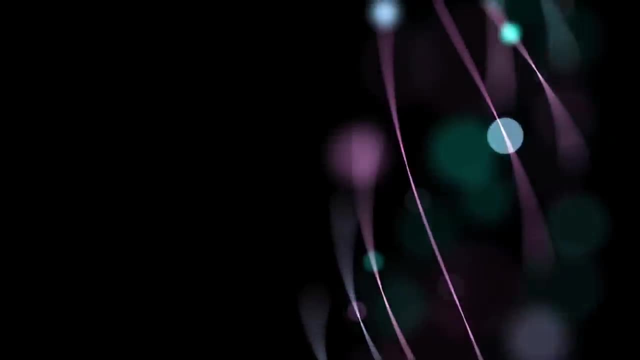 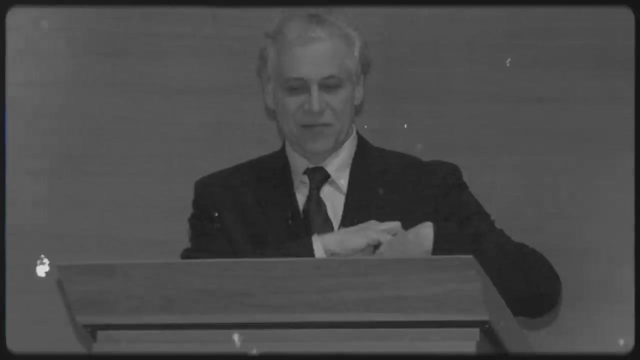 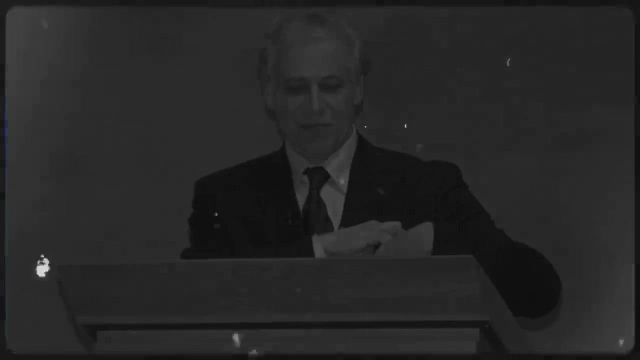 false starts, missed opportunities and nearly ruined careers. Gabriele Veneziano's discovery of a connection between a 200-year-old mathematical formula and the strong nuclear force data was a significant early development in string theory. Leonard Susskind, Holger Nielsen and Yoichiro Nambu. 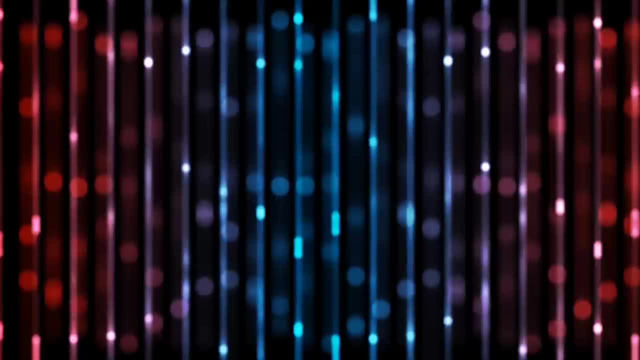 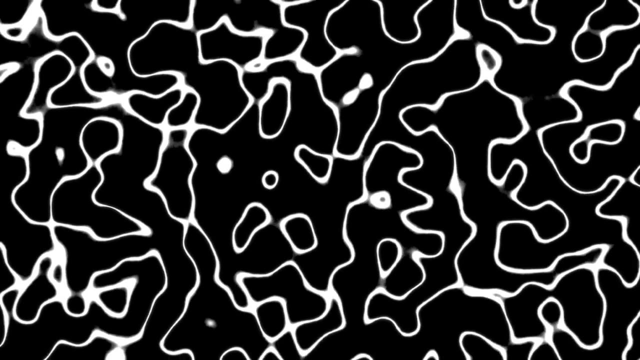 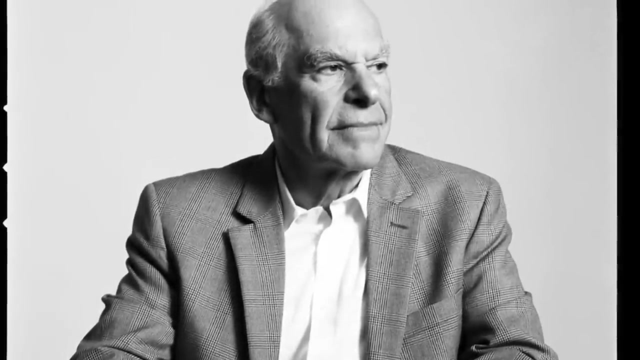 provided the physical underpinnings of Veneziano's discovery leading to the birth of string theory. This theory faced initial skepticism and was overshadowed by quantum chromodynamics, a more conventional theory. John Schwartz and Joel Shirk proposed that string theory could describe gravity as a quantum mechanical theory. 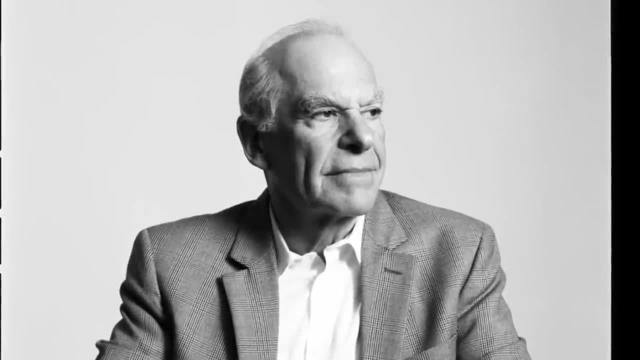 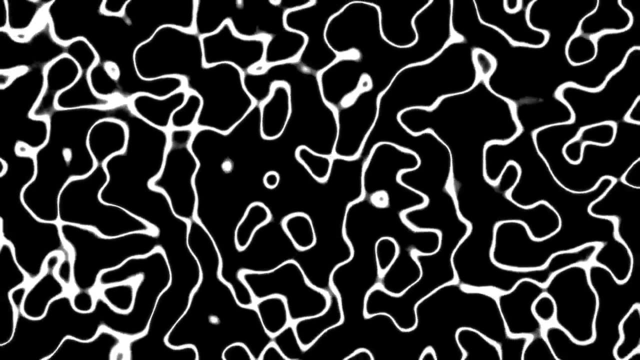 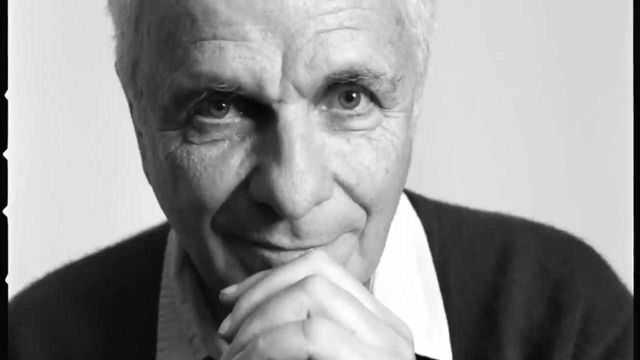 and linked it to the graviton, a massless spin-2 particle. String theory initially struggled due to technical challenges, mathematical inconsistencies and the need for string sizes on the order of the Planck length, making experimental testing impossible. Michael Green and John Schwartz tackled the problem of anomalies in string theory. 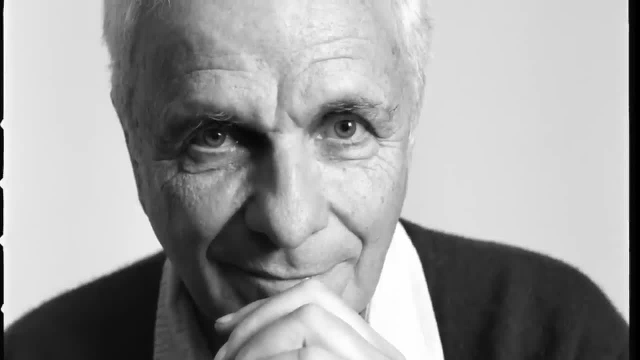 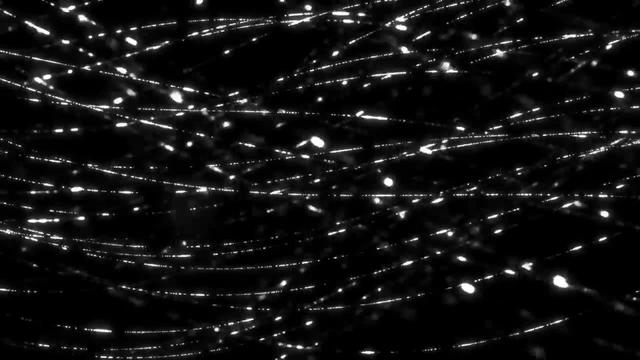 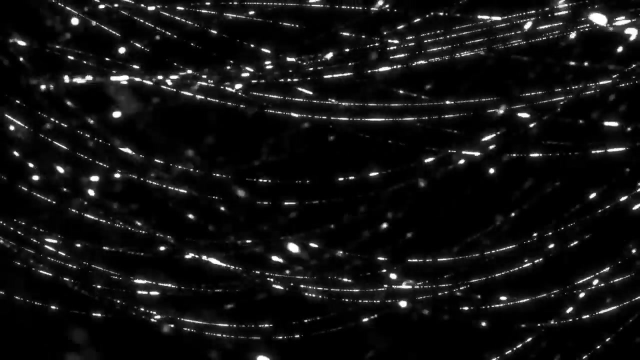 and by 1984, they proved that all potential anomalies cancelled each other out, making string theory mathematically consistent. The acceptance of string theory gained momentum in the mid-1980s as physicists were ready to address the challenge of merging general relativity and quantum mechanics. 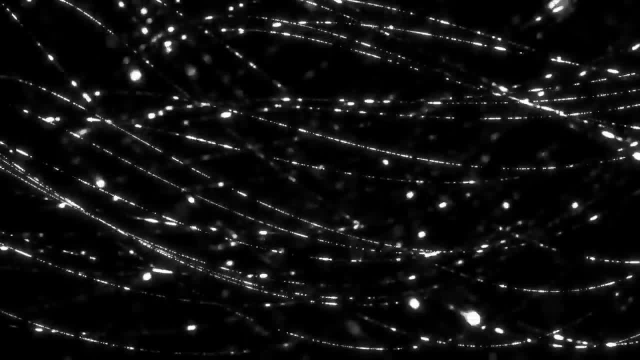 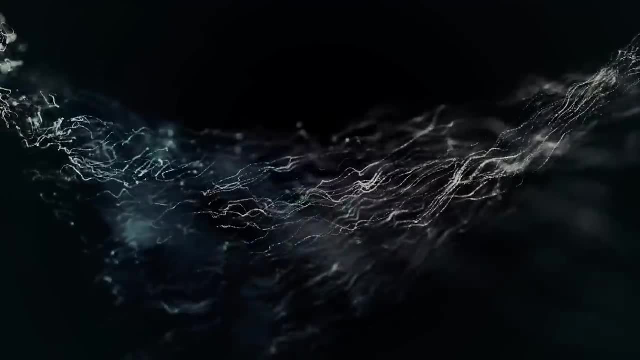 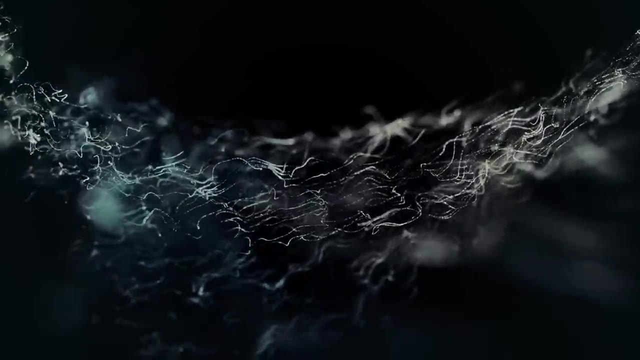 In 1984, a physics revolution was underway and talk of new breakthroughs was spreading rapidly. in the academic community, String theory was a central topic of discussion and its basic ideas were introduced to students and researchers. It was seen as a potential game-changer in physics. 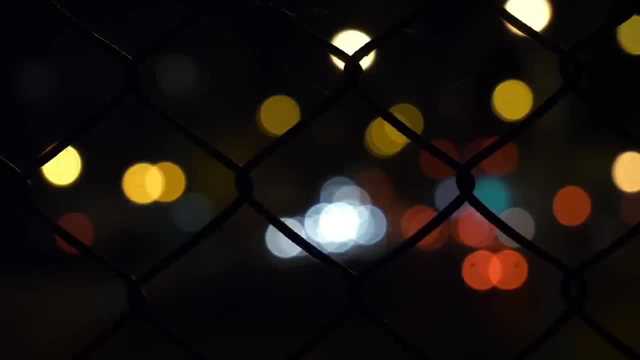 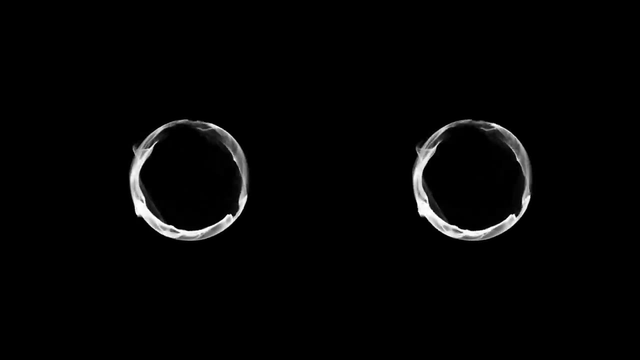 This theory challenged the conventional view of matter by proposing that electrons and quarks are not zero-sized particles, but tiny vibrating filaments of energy called strings. These strings were described as one-dimensional entities with no thickness, only length, and were incredibly small. 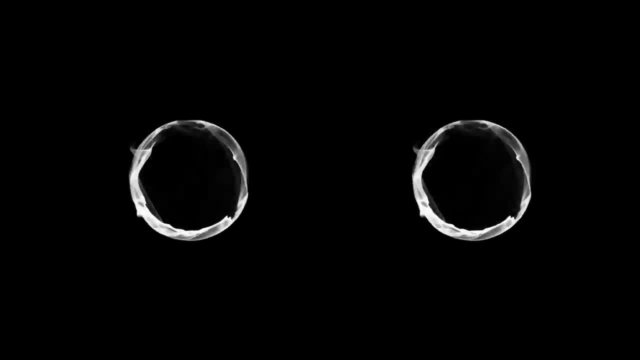 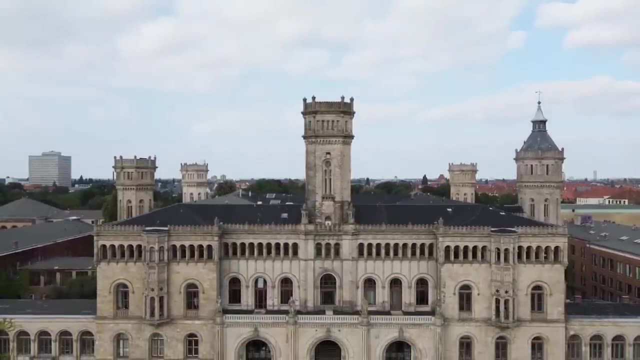 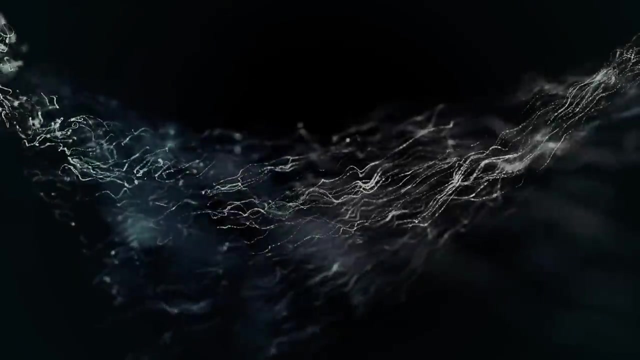 appearing as points, even when examined with advanced technology. The passage acknowledges that string theory's understanding was incomplete, leaving open the possibility that strings might themselves be composed of finer ingredients For the purpose of historical development. the passage assumes that strings are the most elementary ingredient in the universe. 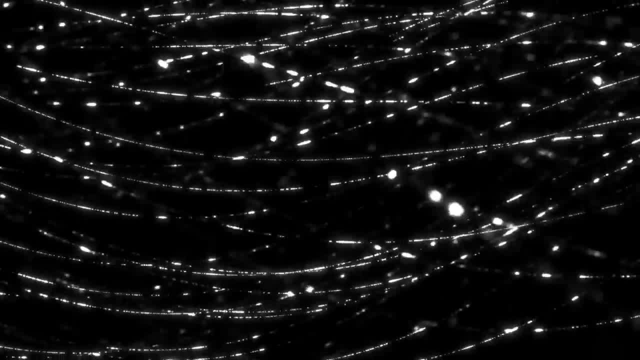 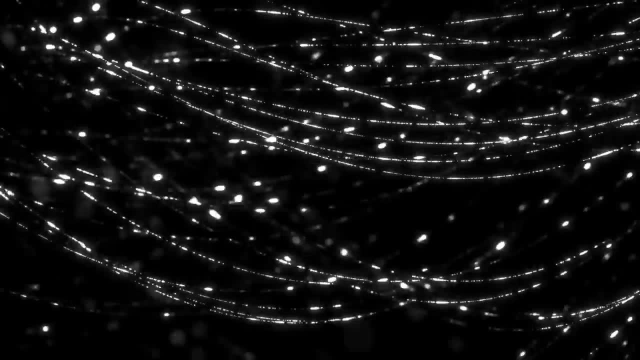 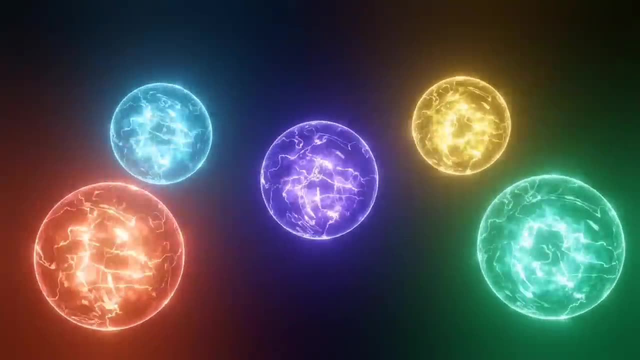 Physicists have spent the past century probing matter to find the universe's elementary constituents. They have discovered particles such as electrons, quarks and neutrinos, which make up ordinary matter. There are different species of quarks, particles similar to electrons, muons and taus. 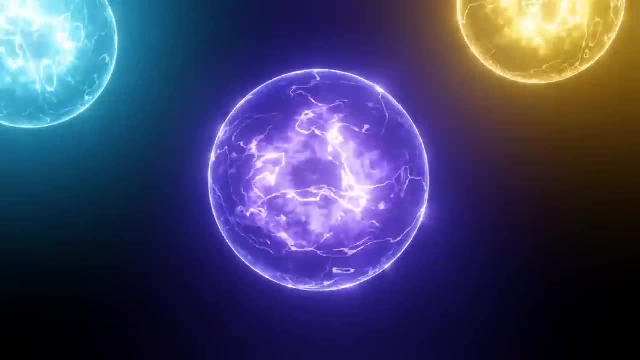 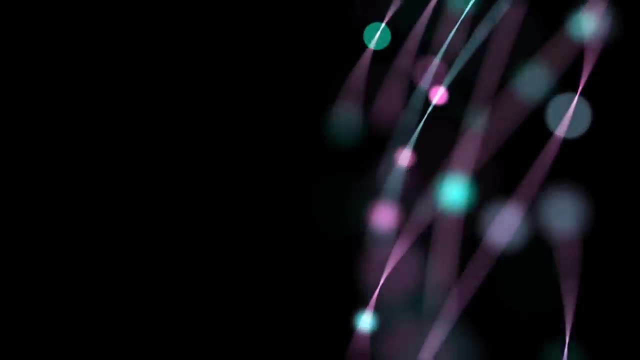 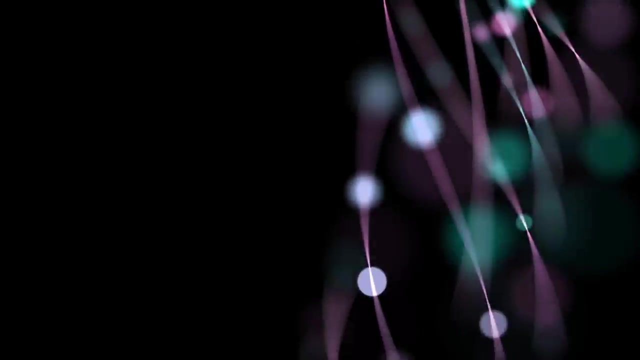 and ghostly neutrinos organized into three families or generations based on increasing mass. String theory proposes that there is only one fundamental ingredient: the string, and the various particle species result from different vibrational patterns of these strings. The vibrational patterns of strings determine the mass. 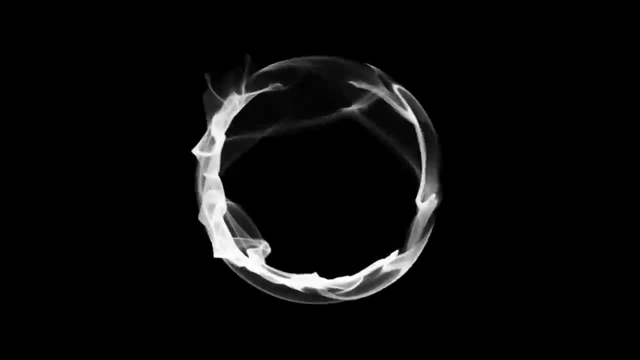 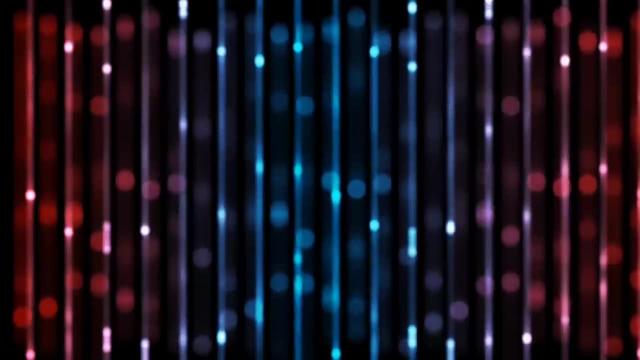 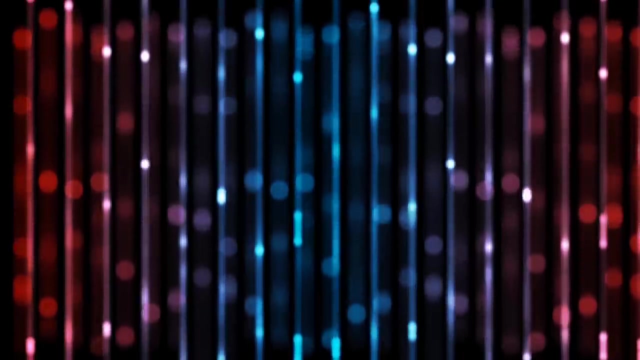 electric charge, spin and other properties of particles. A single species of string can give rise to a variety of particles. It offers a potential unification framework by explaining the particles in terms of vibrational patterns of a single basic ingredient akin to a string symphony: vibrating matter into existence. 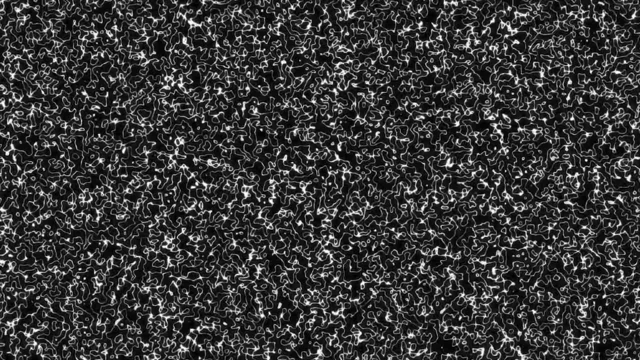 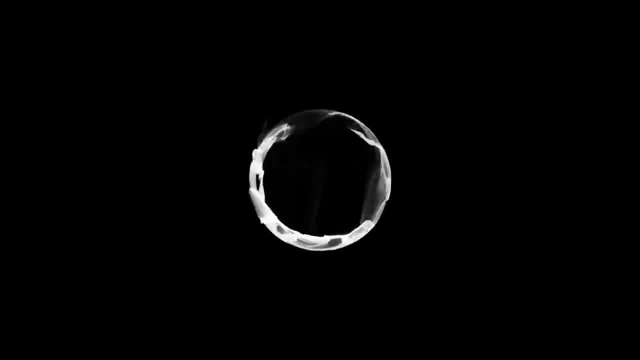 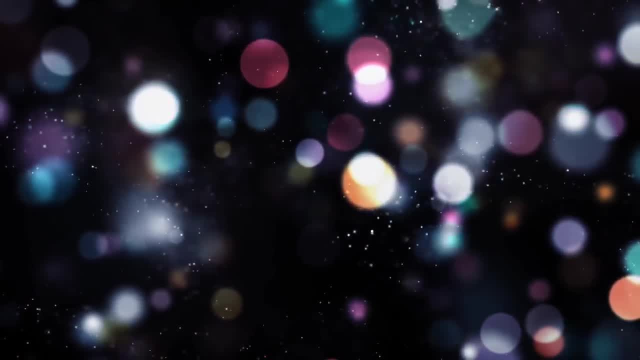 This extends this unification to the messenger particles that transmit the fundamental forces of nature, such as gluons for the strong force and gravitons for gravity. The graviton, a messenger particle for gravity, is incorporated into string theory's quantum mechanical framework. 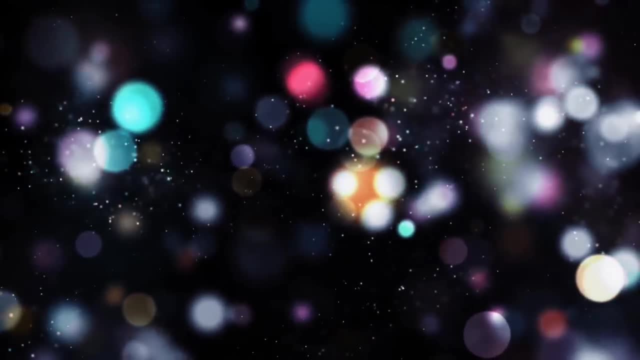 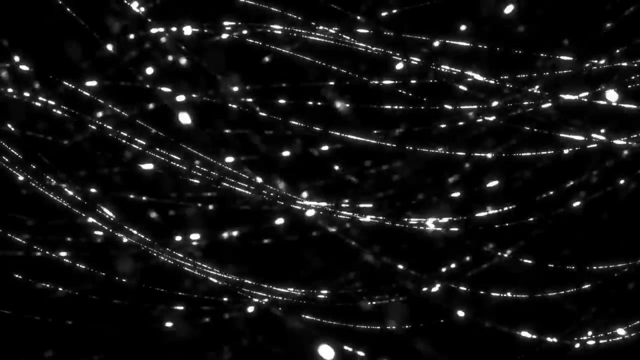 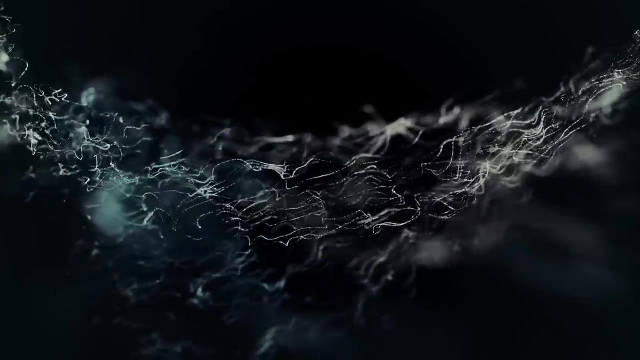 making it a candidate for unifying all forces. String theory's claim of unifying all matter and forces was groundbreaking and gained widespread attention among physicists in the mid-1980s. String theory succeeds in merging gravity and quantum mechanics by introducing strings as its fundamental ingredient. 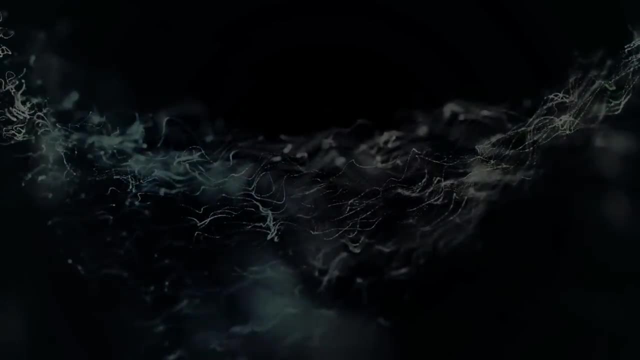 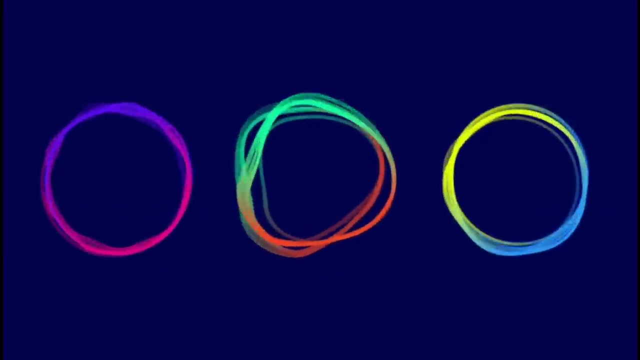 which have spatial extent in contrast to point particles. String theory explains particle properties, including mass, electric charge and spin through the vibrational patterns of strings. Mass corresponds to the energy of a vibrating string with heavier particles, having strings that vibrate faster and more intensely. 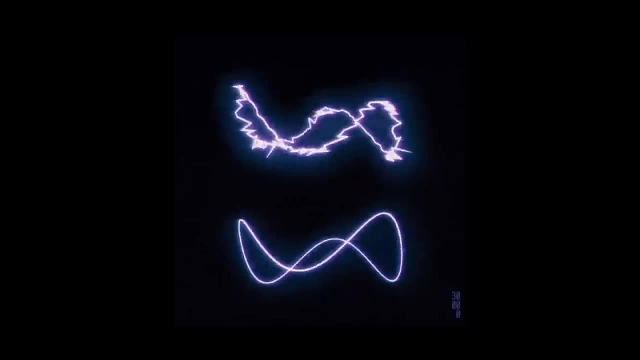 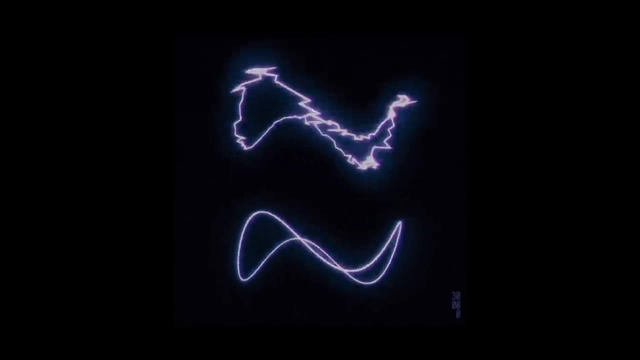 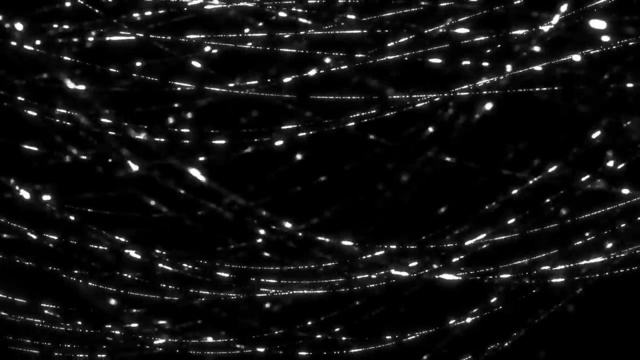 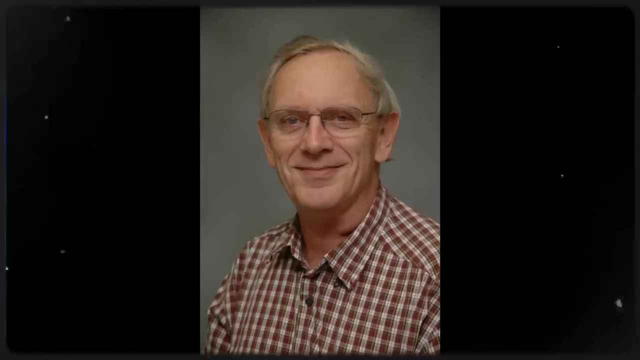 Other properties like electric charge and spin are encoded in more complex features of the string's vibrations. Early bosonic string theory encountered a problem as all vibrational patterns had whole number spin values, while particles of matter had fractional spin. Pierre Ramond and other physicists 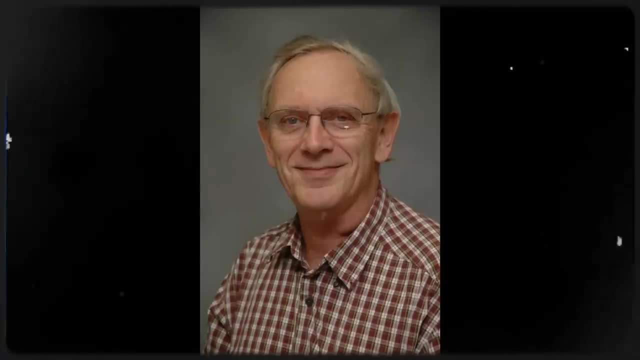 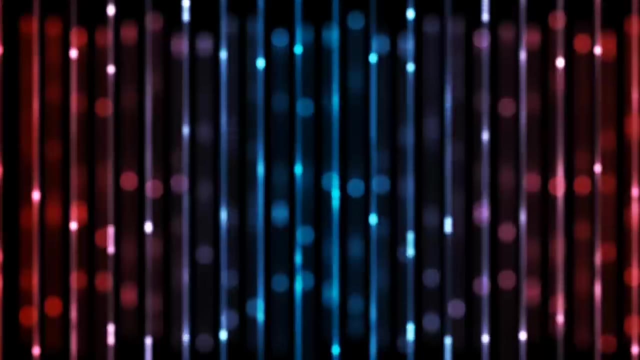 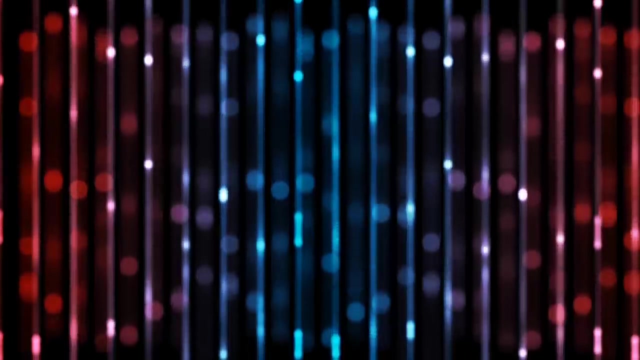 found a way to modify the theory to incorporate half-integer spin values, giving rise to supersymmetry and the birth of superstring theory. For this theory to be viable, its vibrational patterns must precisely match the properties of known particles, as summarized in tables. 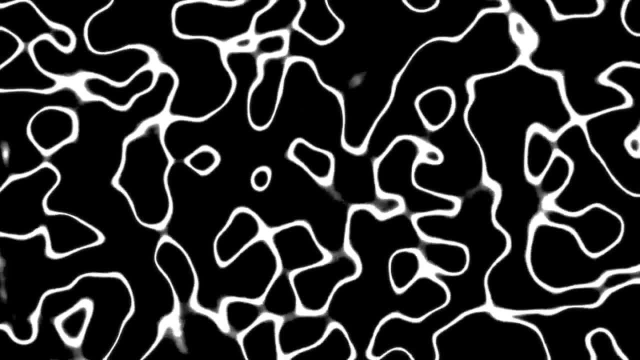 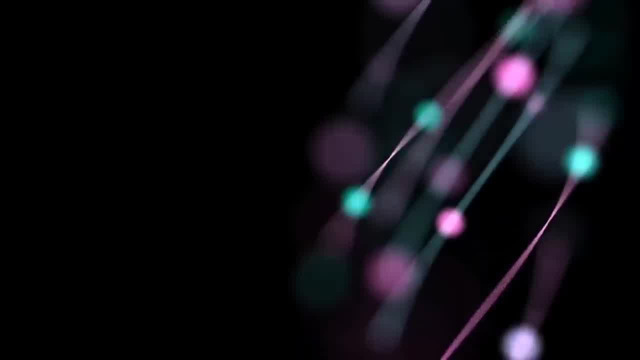 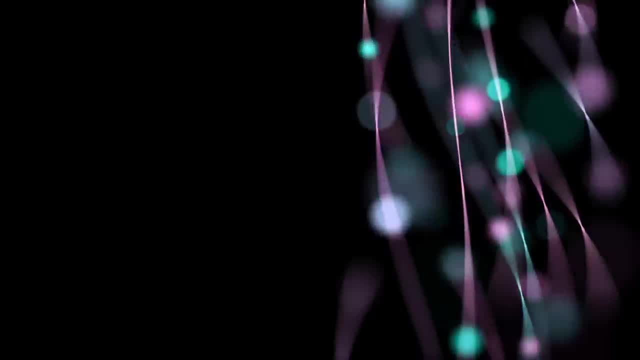 If this match occurs, string theory could provide a fundamental explanation for the universe's particle properties, establishing itself as a unified theory, understanding why the universe is the way it is. String theory faces significant challenges when it comes to matching the vibrational patterns of strings. 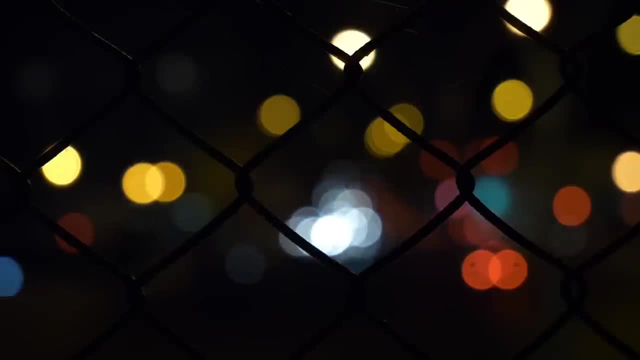 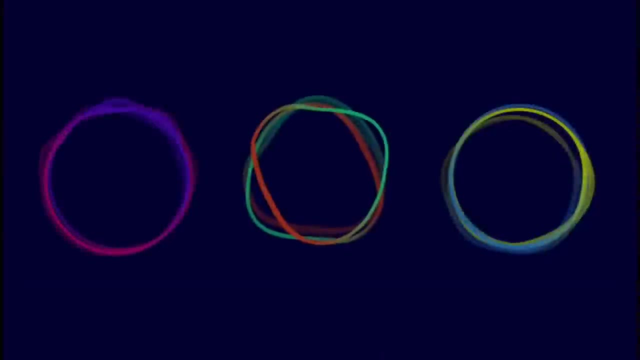 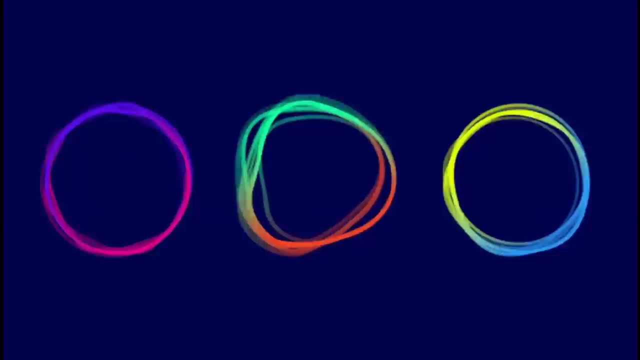 with the properties of known particles, The vibrational patterns can lead to particles with masses that are far too large, as most vibrational patterns are highly energetic, corresponding to particles with gargantuan masses, While the known particle species have some massless particles. 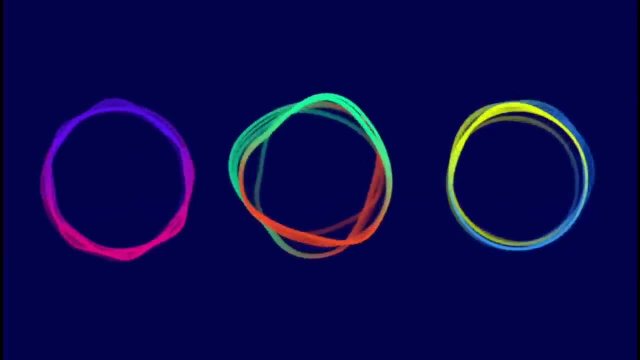 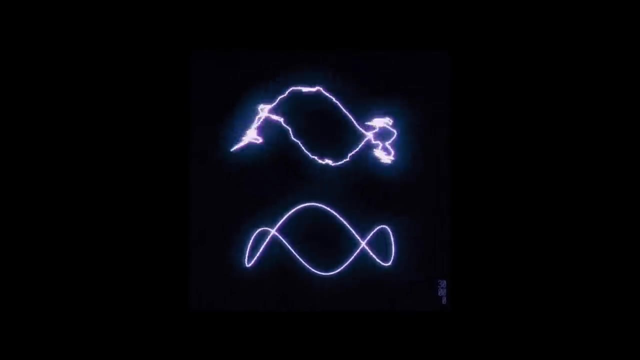 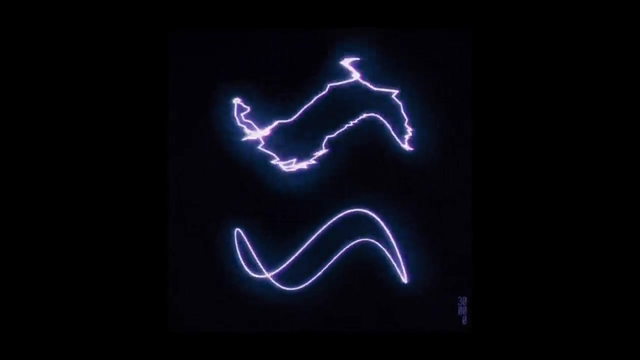 the masses of the permissible string vibrational patterns do not match the experimentally measured particle masses. However, string theory predicts a tower of super-heavy particles and because these would be unstable and decay into lighter particles, they may not have survived to be observed. 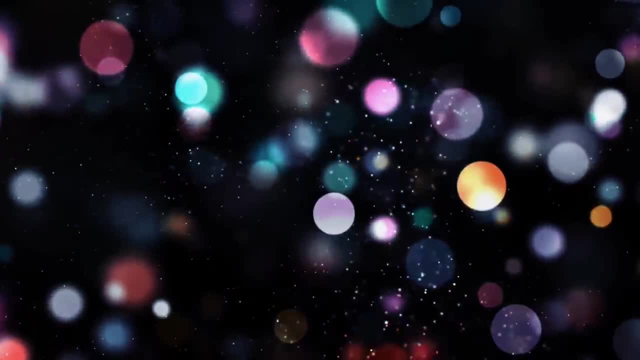 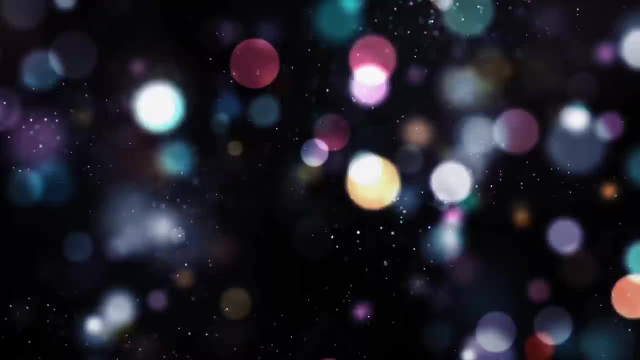 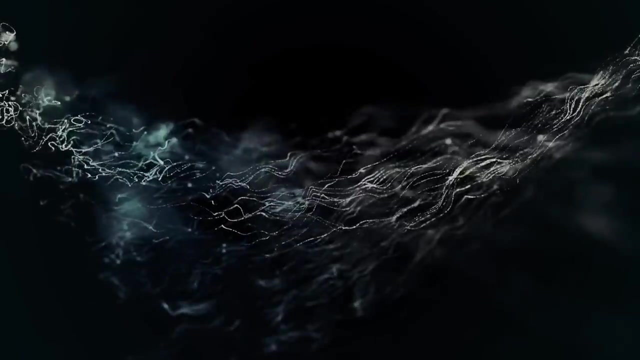 Additionally, current particle accelerators cannot reach energies high enough to excite these super-heavy vibrational patterns. Furthermore, the masses of known particles, although not exactly zero times the Planck mass, are still very close to it. Most particles have masses that are a tiny fraction of the Planck mass. 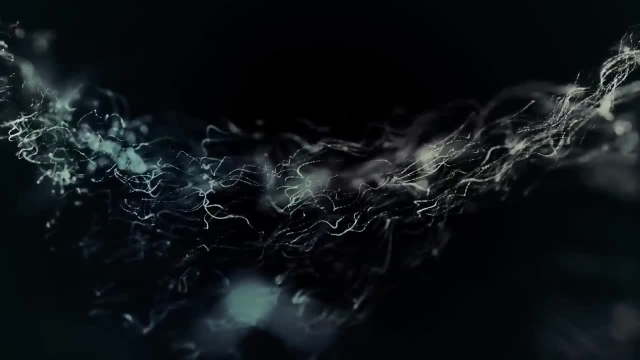 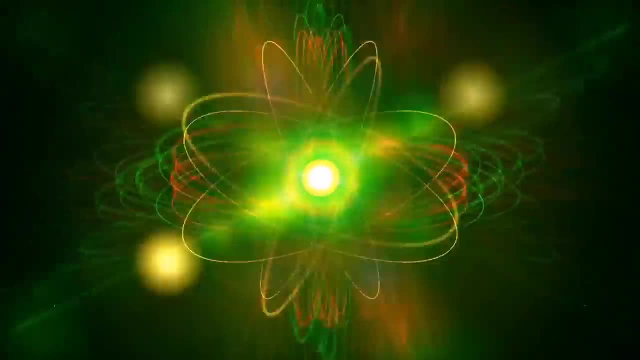 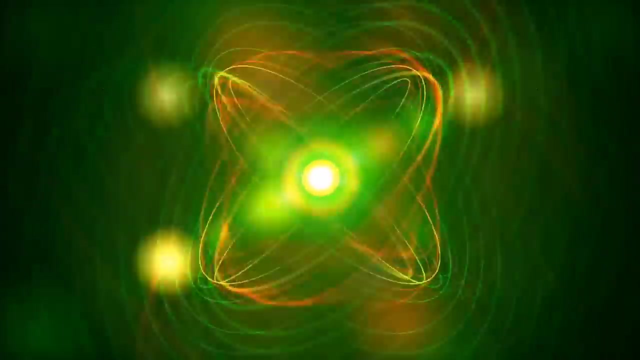 so they can be considered effectively massless within the accuracy of current measurements. Despite these challenges, string theory has promising strategies to overcome them, and it can potentially explain the tiny deviations from zero mass characteristic of known particles. The theory's ability to provide a consistent framework. 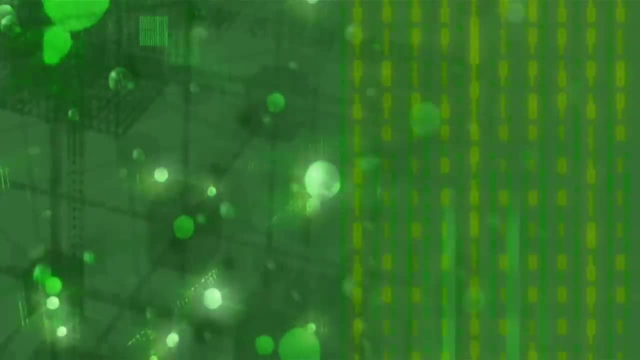 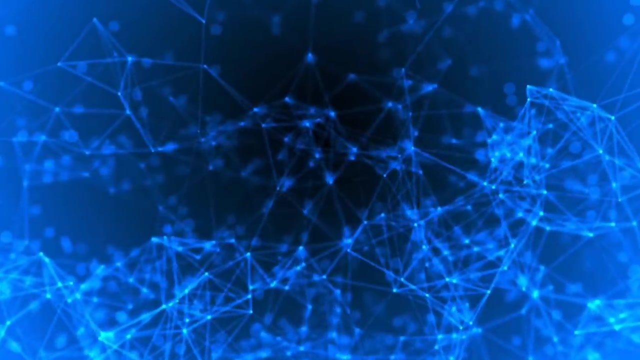 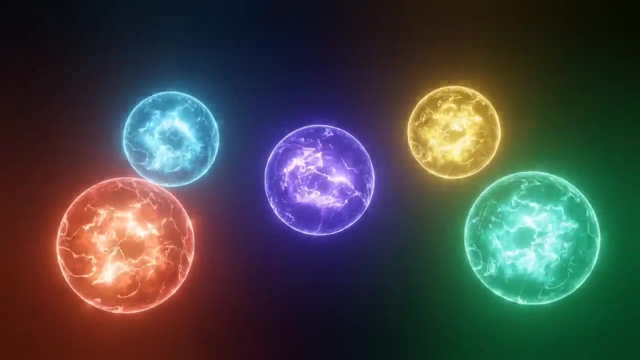 for merging gravity and quantum mechanics is a significant achievement. One major issue is that super-string theory, which is the most promising version of string theory, initially requires ten spacetime dimensions, including nine spatial dimensions. This may seem problematic, but physicists have developed theoretical frameworks. 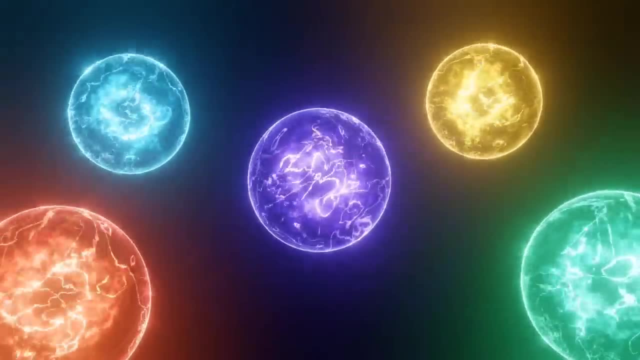 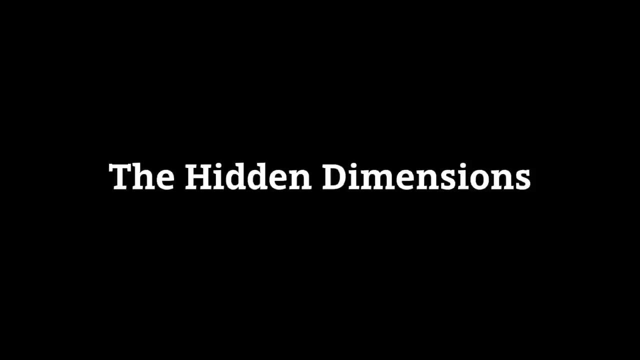 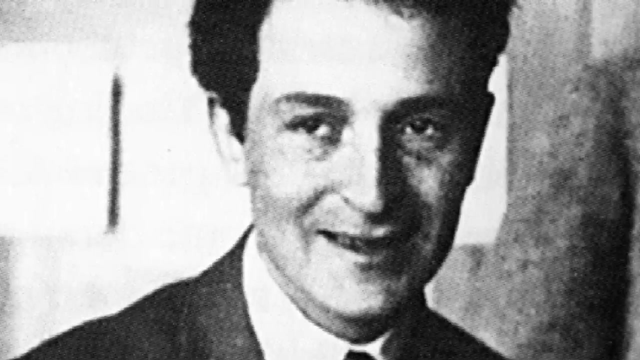 to reconcile these extra dimensions with our observed three spatial dimensions, showing that extra dimensions need not be a problem. In 1919, Theodor Kaluza, a relatively unknown German mathematician, sent a paper to Albert Einstein proposing a radical idea to unify gravity and electromagnetism. 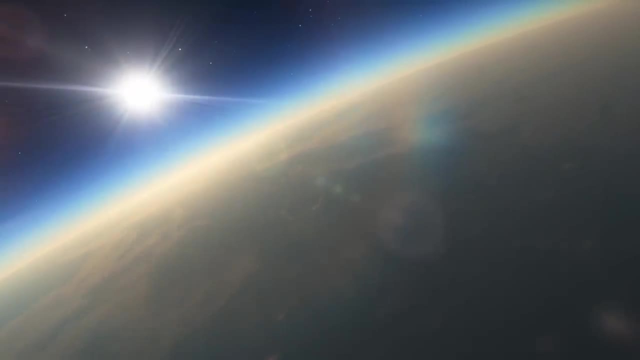 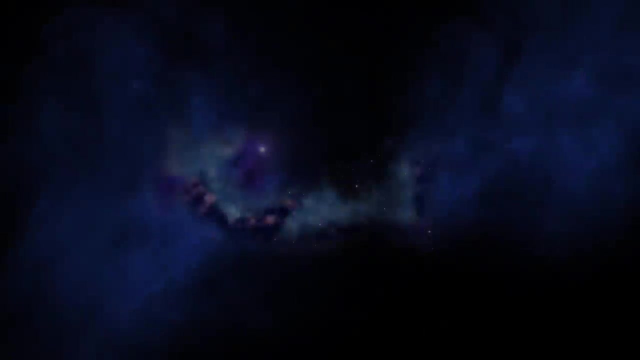 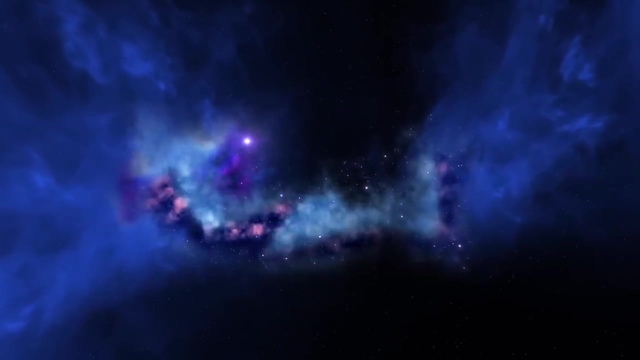 Kaluza suggested that the universe has more than the familiar three space dimensions. It has a total of five spacetime dimensions, including time. In a universe with three space dimensions, any location can be specified with three pieces of information: left right, back forth and up down. 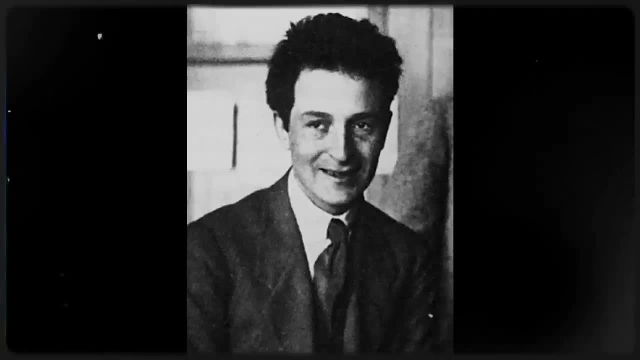 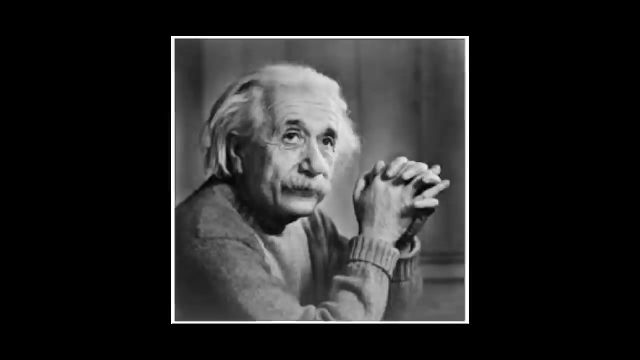 Kaluza proposed the existence of an additional spatial dimension that no one had ever observed, adding a fourth independent direction in which objects could move. The extension of Einstein's equations to include this extra dimension naturally led to additional equations that matched those describing the electromagnetic field. 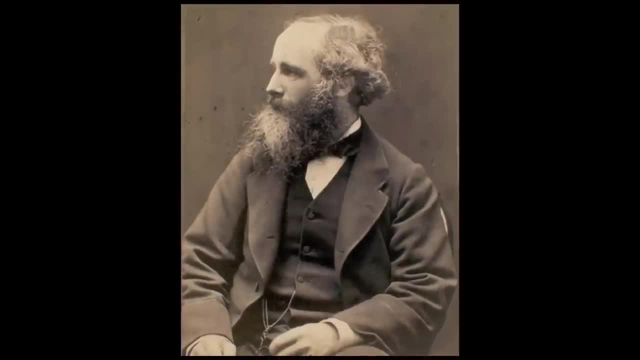 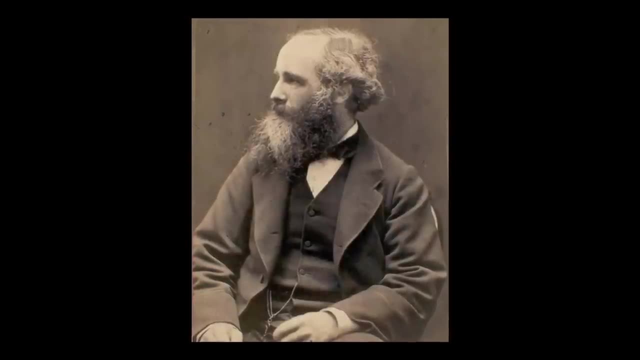 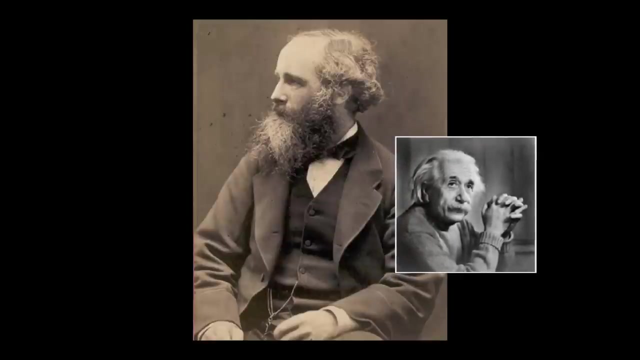 discovered by James Clerk Maxwell in the 19th century. Kaluza's proposal essentially combined Einstein's theory of general relativity, which described gravity, with Maxwell's equations which described electromagnetism in a higher dimensional framework. The mathematics supported this unification. 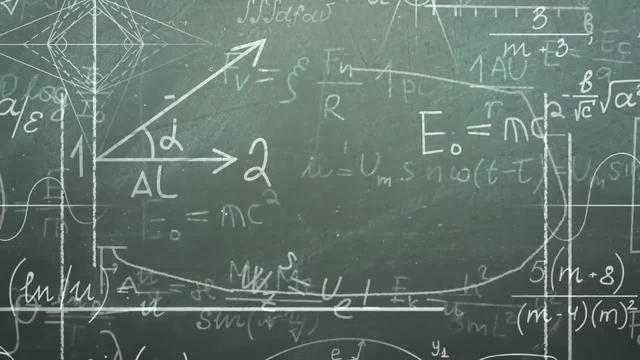 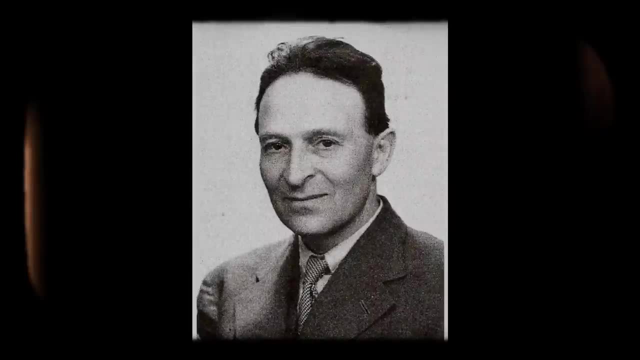 but there was no empirical evidence for an extra dimension at the time. Oskar Klein, a Swedish physicist, in 1926, added a twist to Kaluza's idea, suggesting a way in which the extra dimension could be hidden: The concept of extra dimensions in physics. 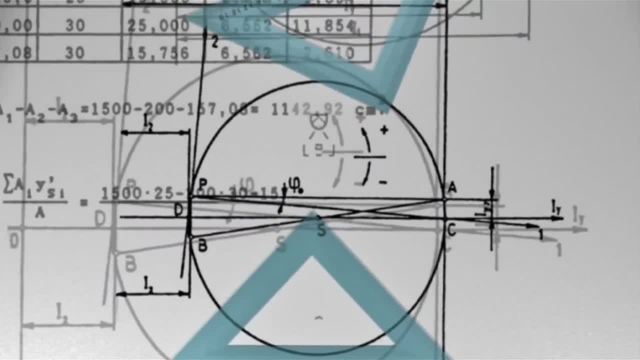 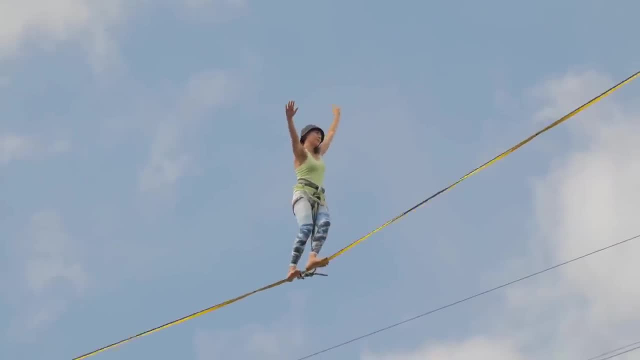 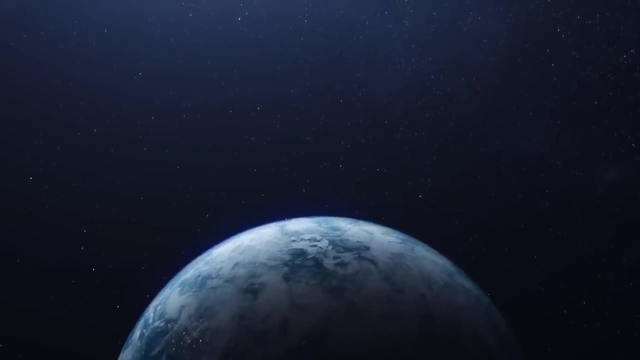 is illustrated using the example of a tightrope with hidden dimensions. Just as a tightrope appears one-dimensional from a distance, but has additional dimensions when closely examined, the fabric of the universe may have hidden small dimensions that are not readily apparent. 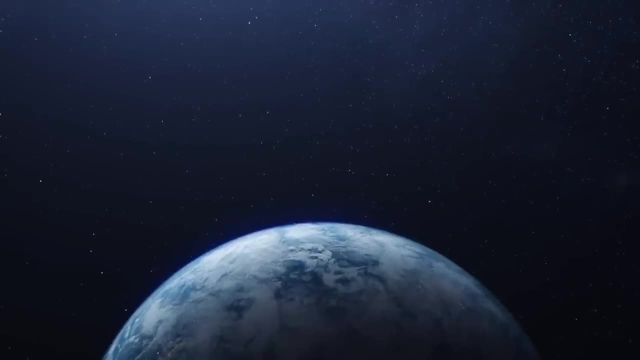 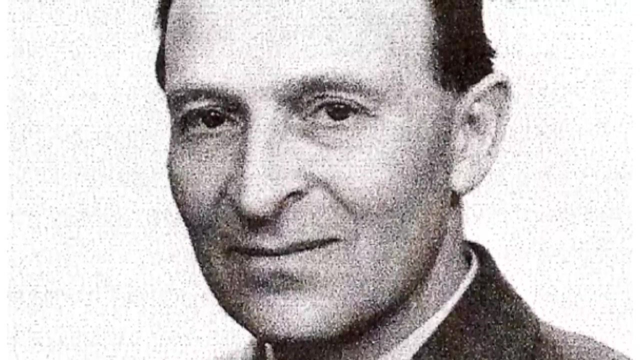 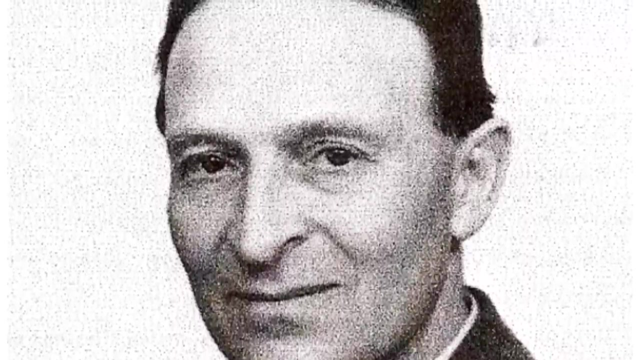 Oskar Klein proposed the idea that the fabric of space itself may have hidden dimensions, similar to how the tightrope has a circular dimension wrapped around it. These hidden dimensions could be as small as the Planck length, making them practically impossible to detect with current technology. 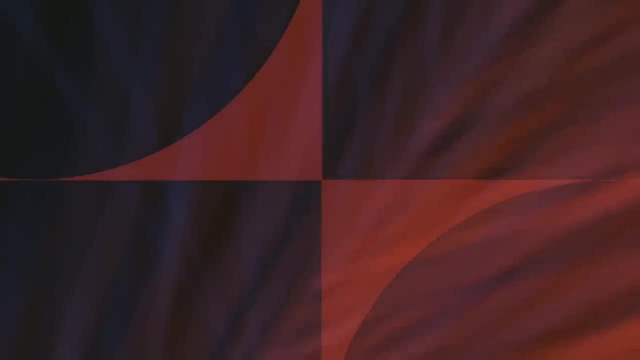 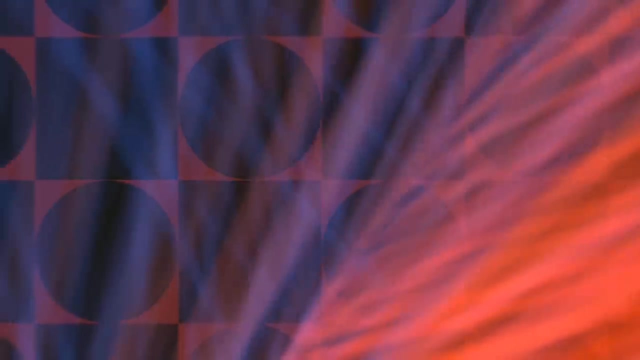 Klein's proposal suggested that these extra dimensions would be present at each point in the familiar three-dimensional space we perceive, just as the circular dimension of the tightrope exists at every point along its length, The addition of these hidden dimensions to the familiar three dimensions of space. 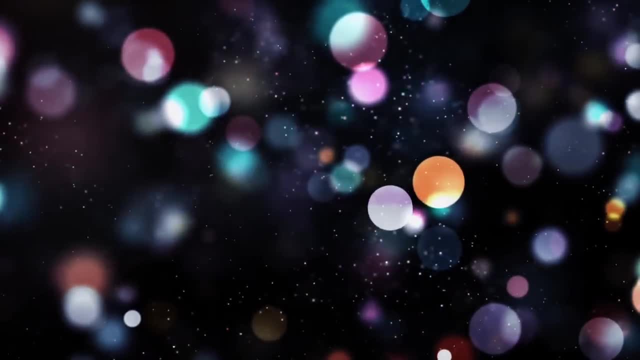 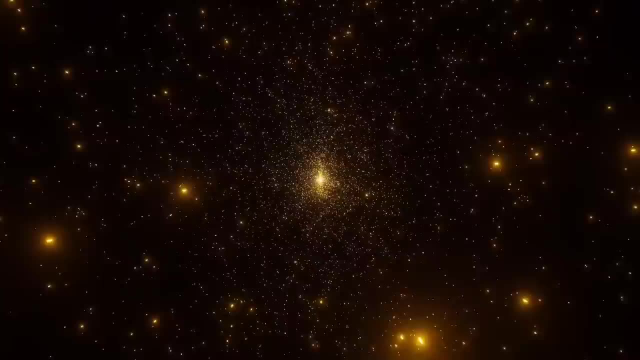 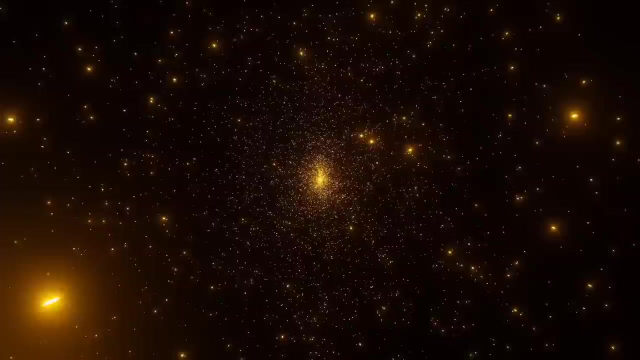 led to the development of Kaluza-Klein theory, which aimed to unify gravity and electromagnetism by introducing extra dimensions. Despite initial enthusiasm, Kaluza-Klein theory encountered difficulties when trying to incorporate particles like electrons into the extra-dimensional framework. and interest in the theory waned for a time. Kaluza-Klein theory would later make a resurgence and become a crucial part of the development of string theory and modern theoretical physics. The original Kaluza-Klein theory introduced the idea of a hidden spatial dimension. 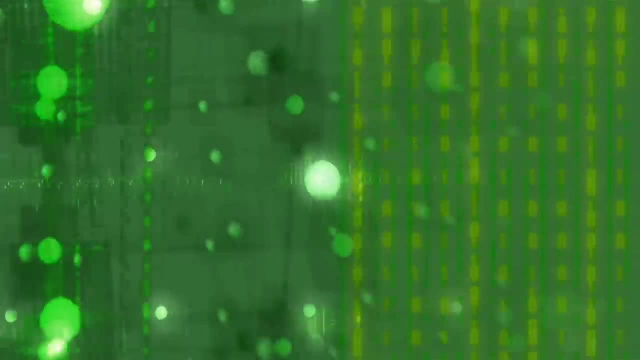 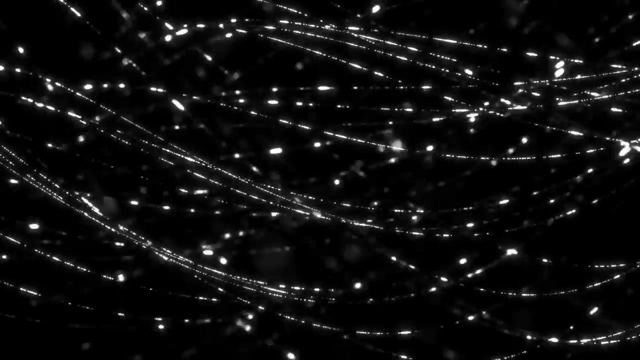 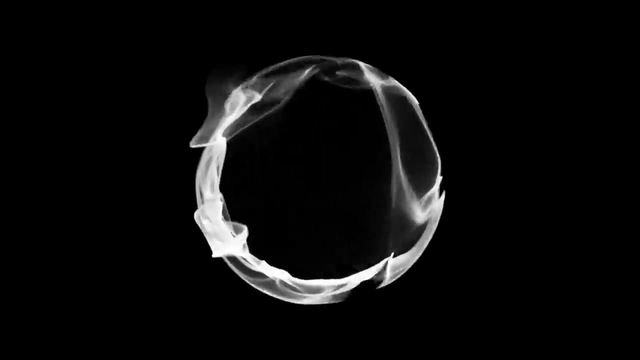 but lacked a convincing reason for why the universe would have exactly four dimensions. String theory is the first theory that predicts the number of space dimensions. It determines that the universe should have ten spacetime dimensions, nine of which are space dimensions. String theory's prediction of ten spacetime dimensions. 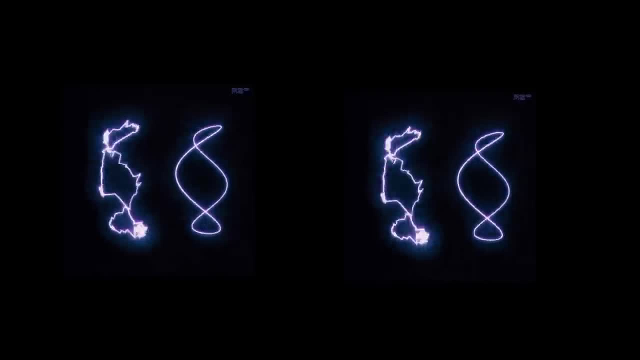 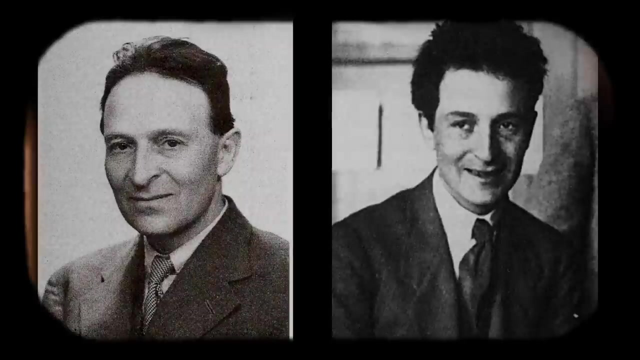 is a calculated result, not an assumption or guess, making it fundamentally different from previous theories. The original Kaluza-Klein theory proposed one hidden dimension, but can be generalized to include more. For instance, it can accommodate two, three or even six extra dimensions. 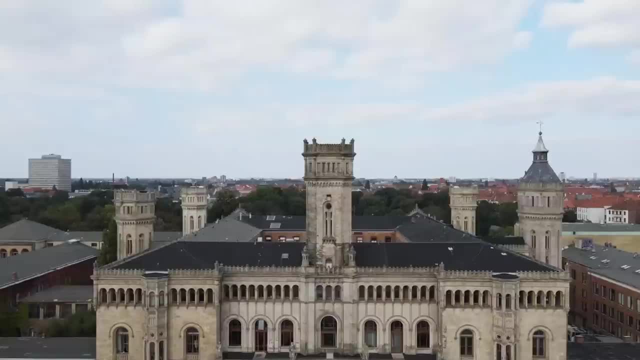 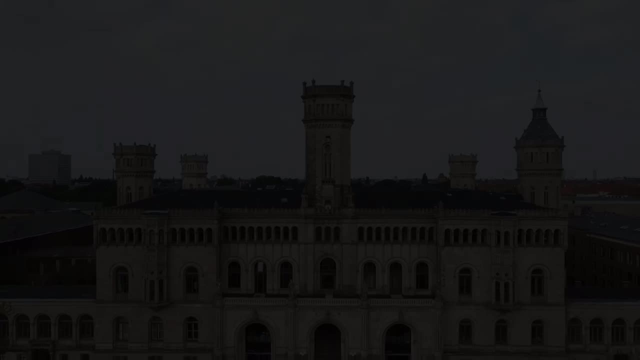 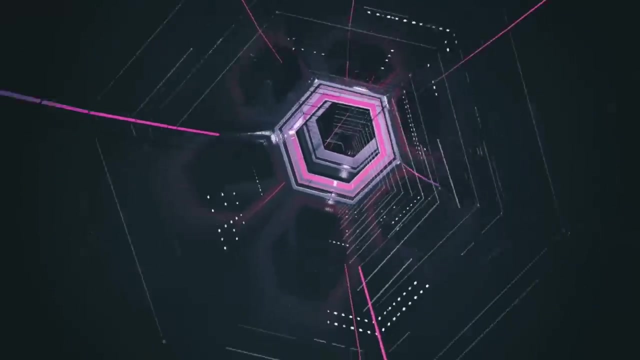 as required by string theory. In a universe with six extra dimensions, specifying a point's location would require nine pieces of information: three for the usual three spatial dimensions and six for the hidden dimensions. The extra dimensions could be so small that they have escaped detection. 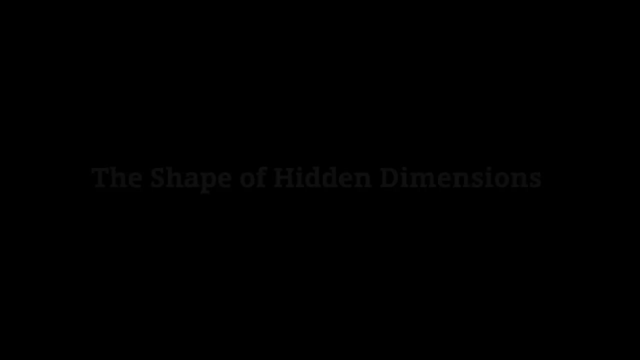 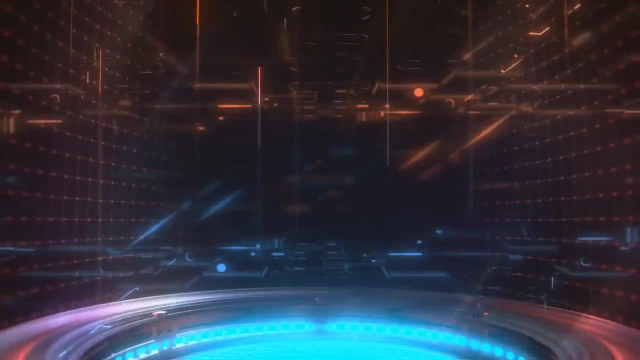 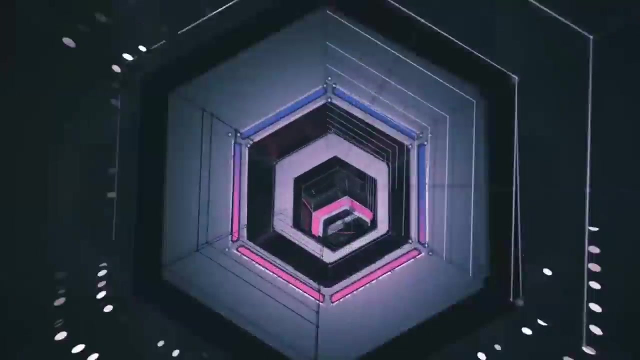 allowing them to remain hidden from our observations. The equations of string theory not only determine the number of spatial dimensions, but also specify the shapes these extra dimensions can take. These extra dimensions are described by complex six-dimensional shapes known as Calabi-Yau spaces. 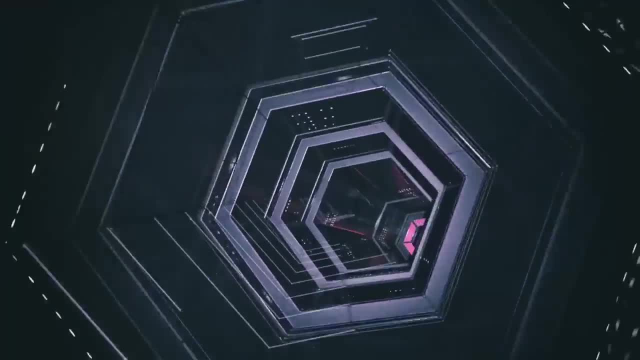 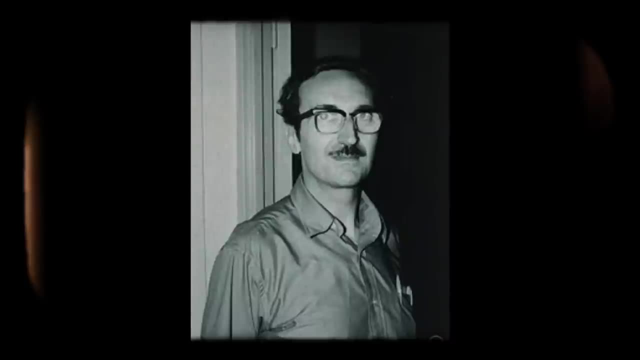 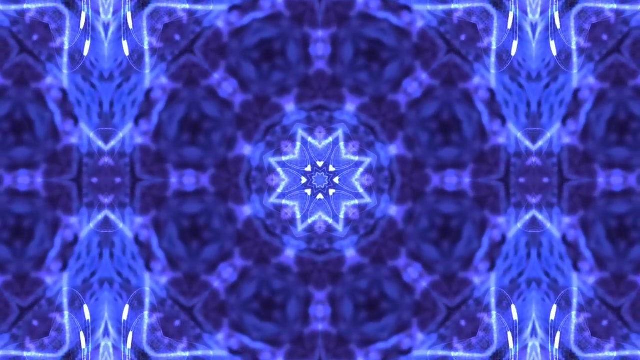 named after mathematicians Eugenio Calabi and Xingtung Yao. Calabi-Yau shapes are highly complex and are difficult to visualize in ordinary three-dimensional space. Imagine if the extra dimensions in string theory were Calabi-Yau shapes On ultra-microscopic scales. 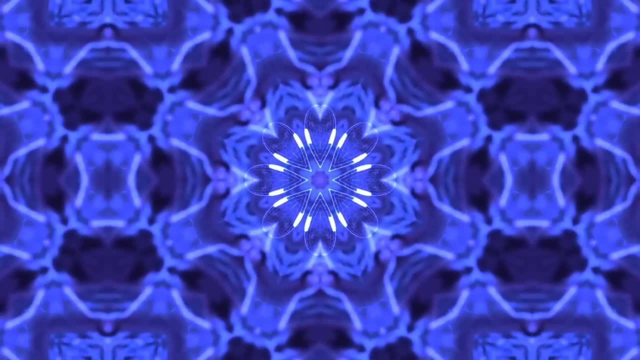 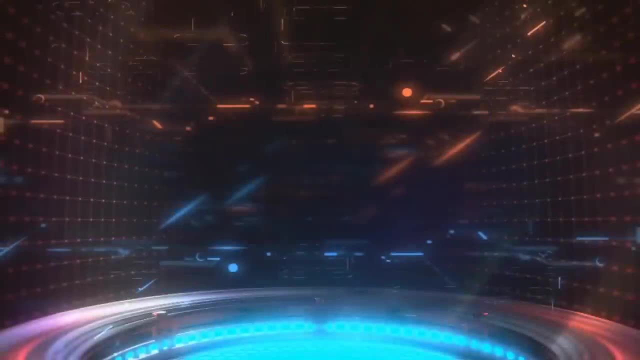 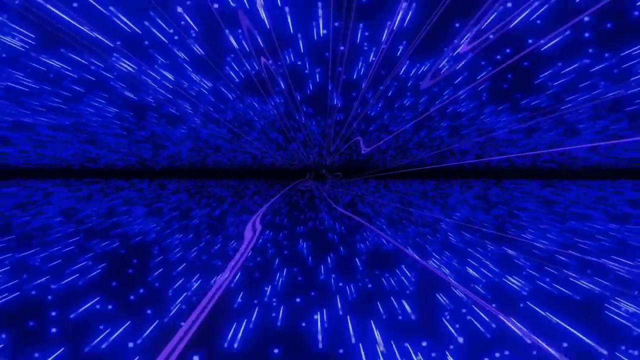 space would be filled with these intricate shapes. As these shapes are tacked onto every point in the usual three dimensions, we would effectively move through all nine dimensions as we go about our daily lives, but we wouldn't perceive these extra dimensions directly. String theory requires ten space-time dimensions. 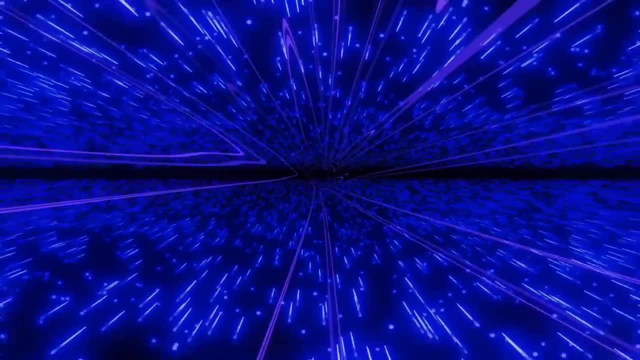 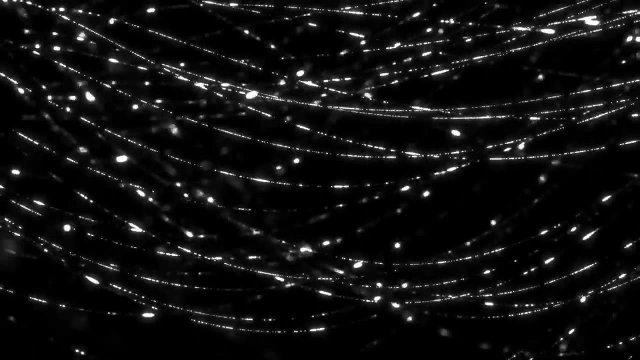 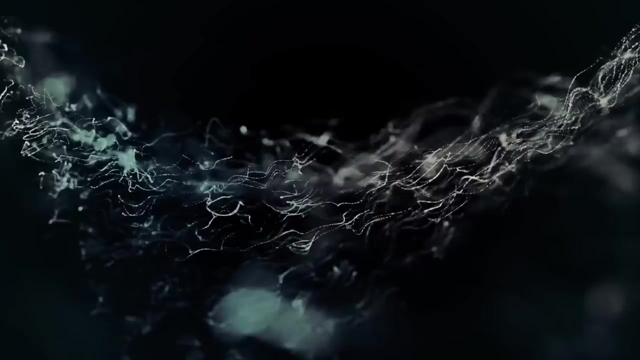 and this arises from an interplay of geometry and physics. More spatial dimensions allow for more vibrational patterns of strings, which are crucial in string theory. The precise size and shape of the extra dimensions influence string vibrational patterns and particle properties. Calabi-Yau shapes are complex six-dimensional shapes. 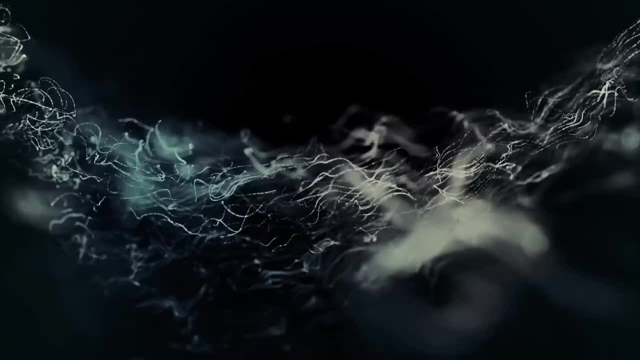 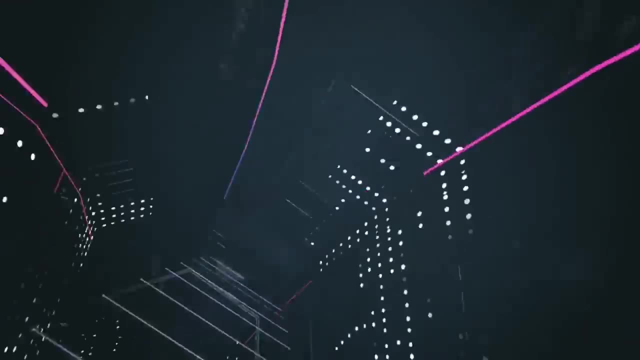 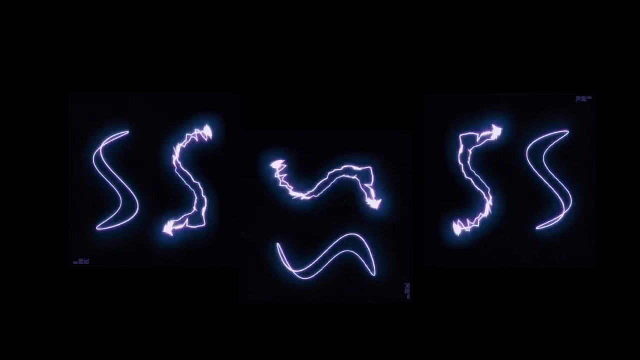 that play a crucial role in determining the properties of string vibrational patterns. The exact choice of Calabi-Yau shape and the size of the extra dimensions are still open questions in string theory, While the exact masses of particles are challenging to calculate in string theory. 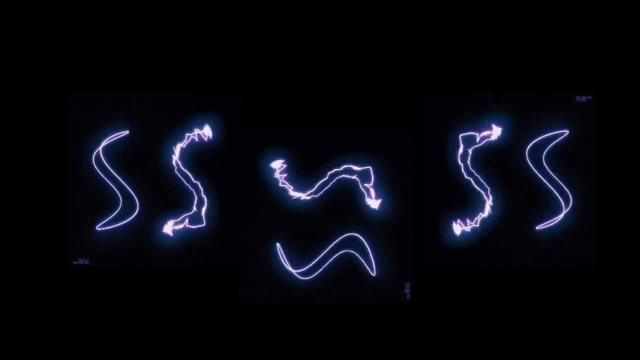 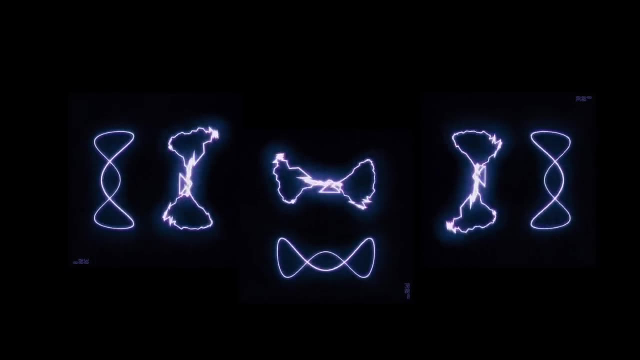 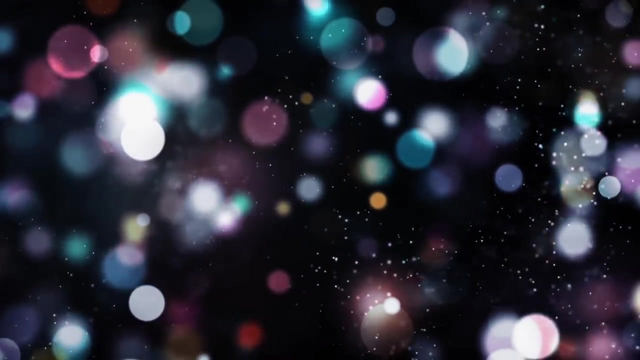 it's possible that tiny masses may arise through interactions between strings, similar to how the Higgs field imparts mass in the standard model of particle physics. String theory holds the potential to explain fundamental particle properties and provide a deeper understanding of the universe. Even though much about string theory 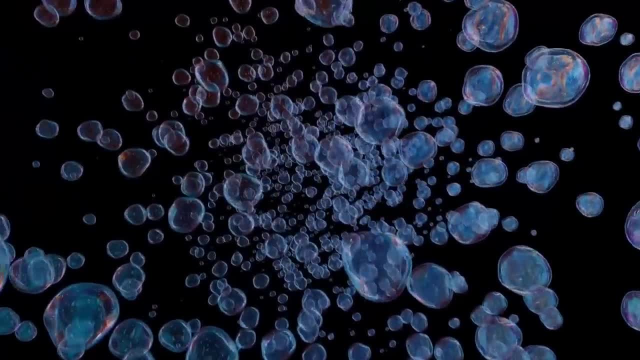 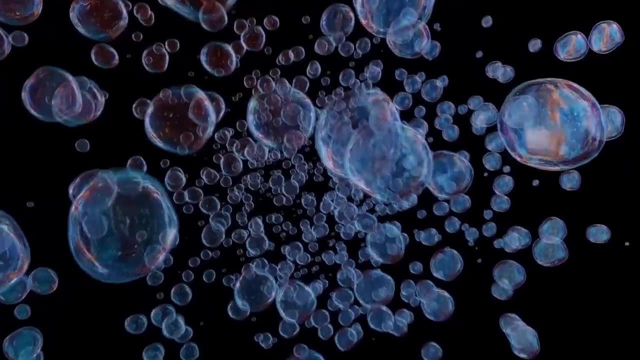 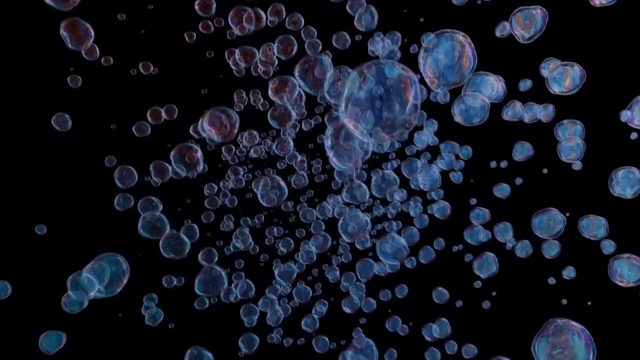 still lies beyond the bounds of our comprehension. it has already exposed dramatic new vistas, Most strikingly in mending the rift between general relativity and quantum mechanics. string theory has revealed that the fabric of the cosmos may have many more dimensions than we perceive directly. 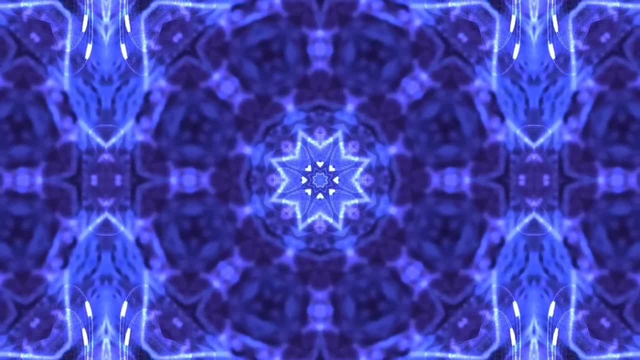 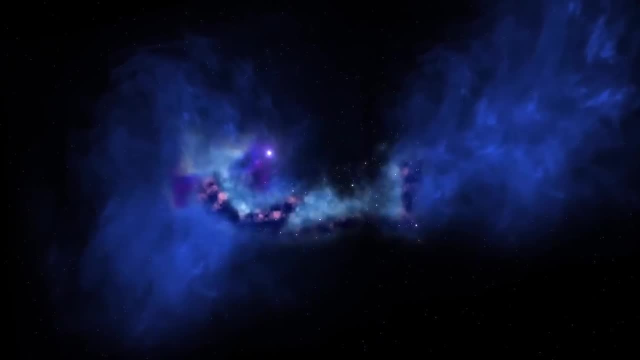 dimensions that may be the key to resolving some of the universe's deepest mysteries. Moreover, the theory intimates that the familiar notions of space and time do not extend into the sub-Planckian realm, which suggests that space and time as we currently understand. 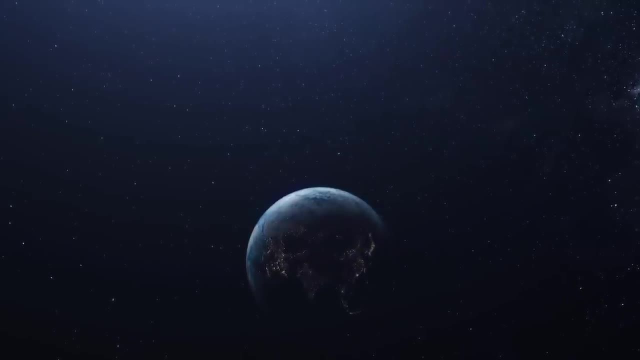 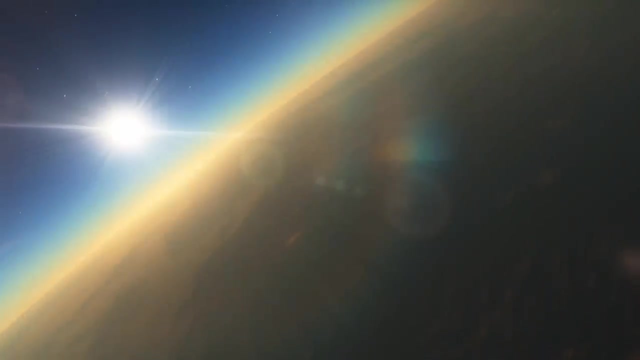 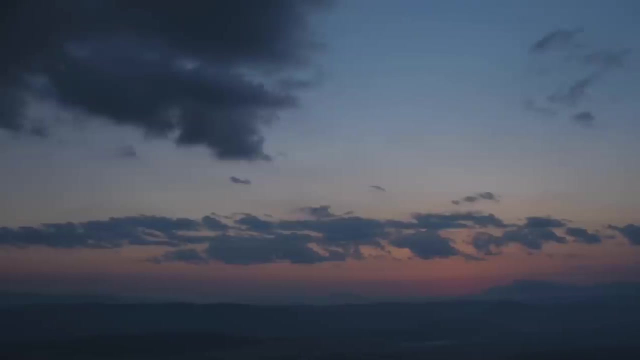 may be mere approximations to more fundamental concepts that still await our discovery. In the universe's initial moments, these features of the space-time fabric that today can be accessed only mathematically would have been manifest Early on, when the three familiar spatial dimensions